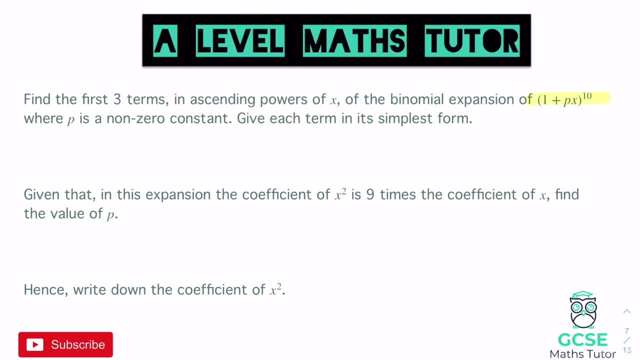 of something like this shown just here: 1 plus px to the power of 10 and obviously looking towards solving a problem to do with that as well. so looking at sort of the coefficients of x squared and trying to solve one of these problems. So this is what we're going to build. 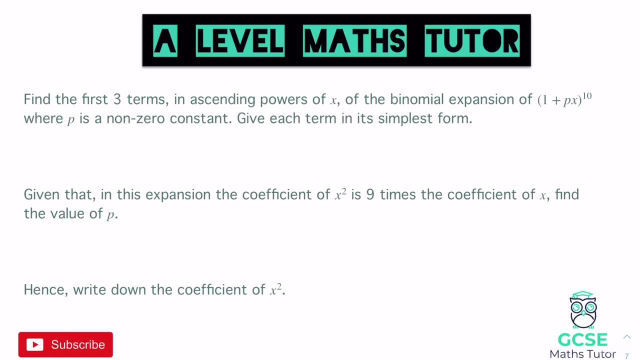 towards. but we're going to start right at the beginning and having a look at binomial expansion right from sort of something that we did at GCSE level and building it right up to one of these more tricky problems. So we're going to get started on one of those. 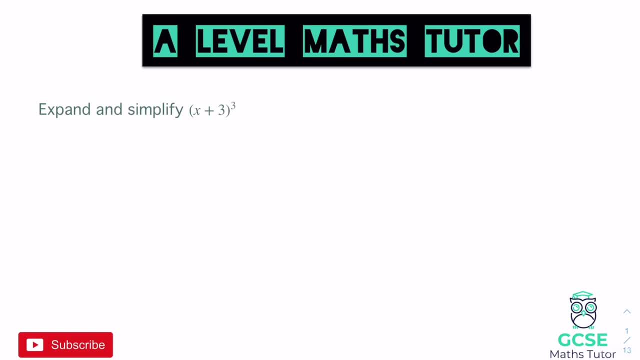 now and here it is Okay. so when we're looking at binomial expansion- essentially we're thinking about from GCSE level, where we've looked at expanding and simplifying a triple bracket- We're going to look at sort of how this all sort of interlinks with then higher powers when we have sort 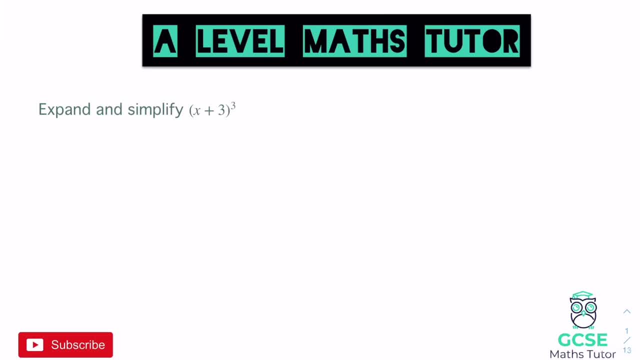 of a bracket to the power of 5 or to the power of 8, and how we go about finding those powers using this process. Now, when it comes to binomial expansion, it's all sort of interlinked with sort of the separate powers. when we've looked at brackets Now, if we think about sort of 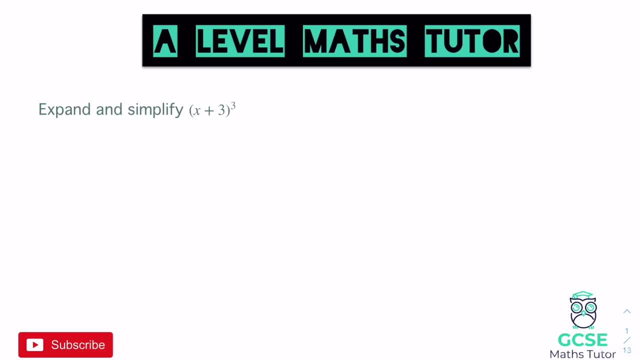 a nice, easy one, something like x plus 5 in brackets It's squared. we get a certain pattern that sort of comes out of these, and when we expand one of these we get the x squared. we get that first piece. there is always to that power. 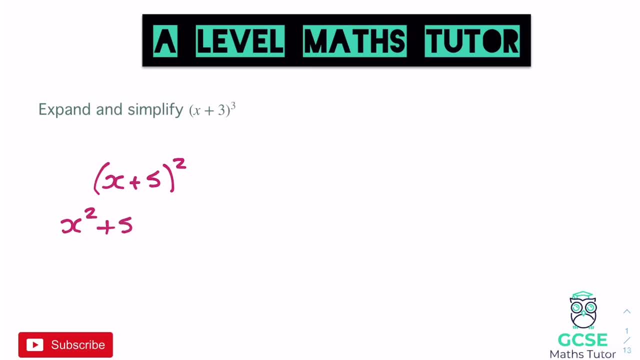 of 2.. Then we get the 2 in the middle, we get plus 5x, plus 5x, and we always get these two there, and then you get that 5 at the end, which is squared as well to make 25.. And then, obviously, 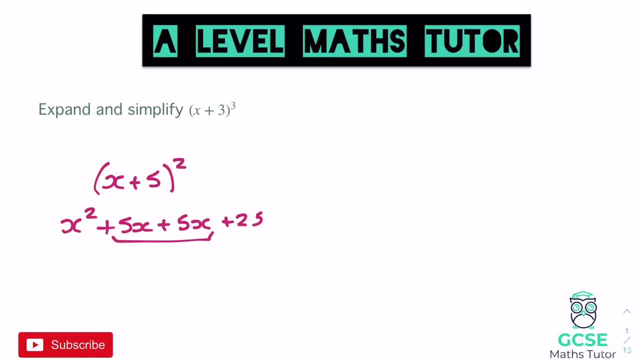 those two in the middle are added together. but we get this sort of little pattern and it's all linked to Pascal's triangle And Pascal's triangle is nice and easy to do. So we draw, we get a 1 at the top, then you add together the numbers either side of it. 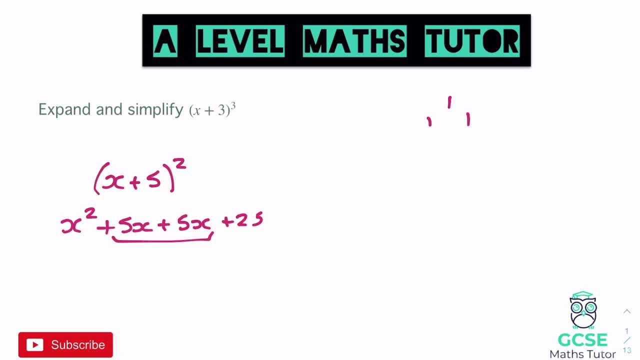 to get the ones below, and obviously 1 at the top has got a 0 either side, so we just have 1 and 1 below that. But then when we add these together we get 1 on the left. those two 1's add to make 2 in the middle and then we get 1 on the end and we can just keep following. 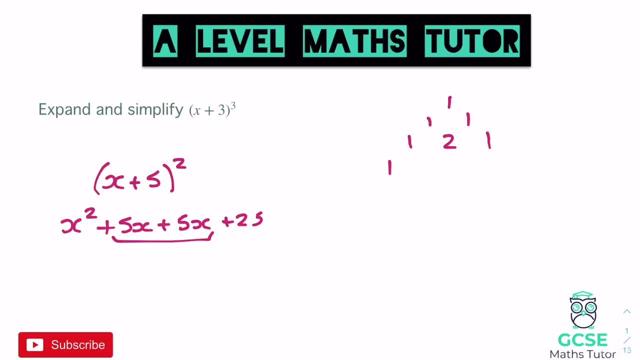 this process and making this pattern so always 1 on the outside, Then the 1 and 2 above this, next one makes 3, 2, and 1 makes 3 and 1, and we can keep on going. 1, 3 and 1 makes 4, 3. 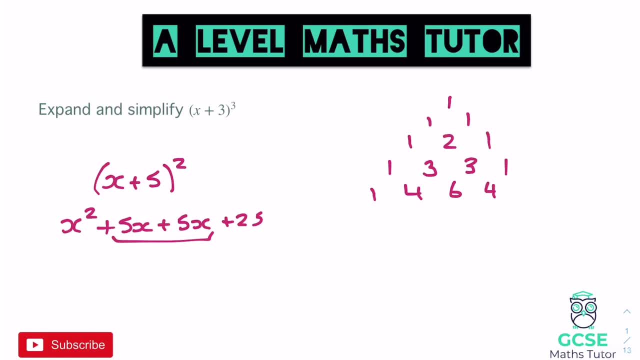 and 3 makes 6.. 3 and 1 makes 4 again, and then 1 at the end, and we can keep on going, basically, with this. Now, when it comes to this double bracket that I've drawn here, that is, this row here, So, 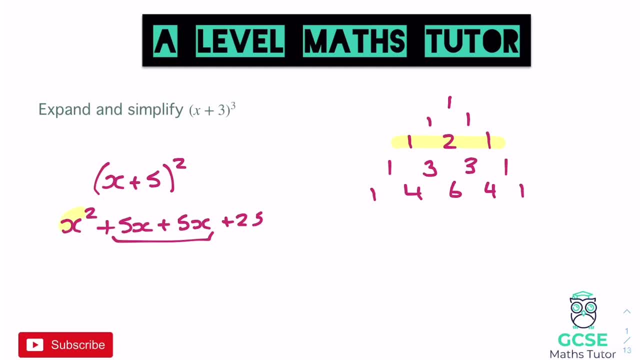 1, 2, 1.. So we get 1 of the pieces at the start, the x squared. We get the two pieces in the middle which we've obviously just shown there. We get the 2 in the middle and then. 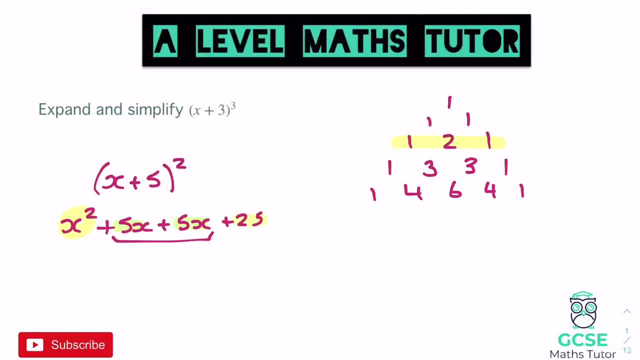 we get the 1 at the end and following that little pattern of 1,, 2, 1.. Now, if I come away from that and we have a look at this triple bracket, which is what we're going to have a look at to start, 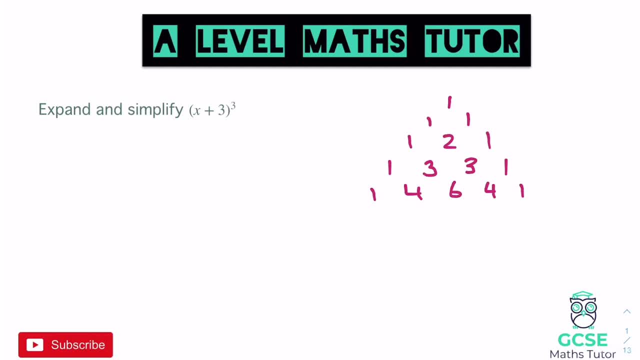 That is obviously linked to the next row down. Now that next row down is 1, 3,, 3, 1.. Now it's not as easy to spot the pattern with this one, but obviously if we were to expand this all and have a look at all the pieces, we would see we get the 1 at the start. We always get. 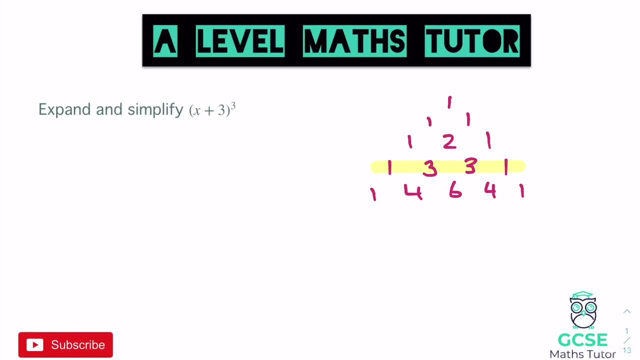 an x cubed at the start. We get the 1 number at the end, which is going to be that 3 cubed which we'll have a look in a sec, And we get these two, lots of the three pieces in the middle and we're going to have a look at those now. 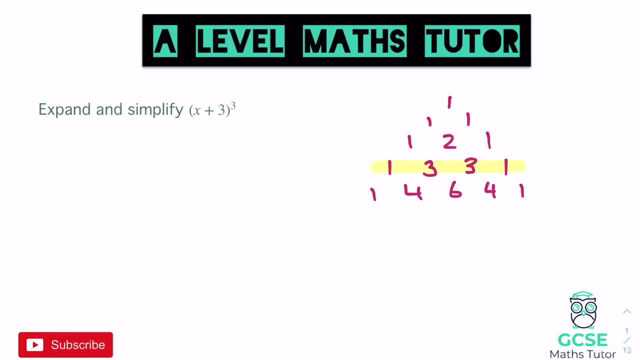 So, if we have a little think, when we were to expand this at GCSE, obviously what we would do is we would expand 2, lots of the 3 pieces in the middle and we would have a look at 2 brackets to start with. So we would do x plus 3 and we're going to fully expand this. 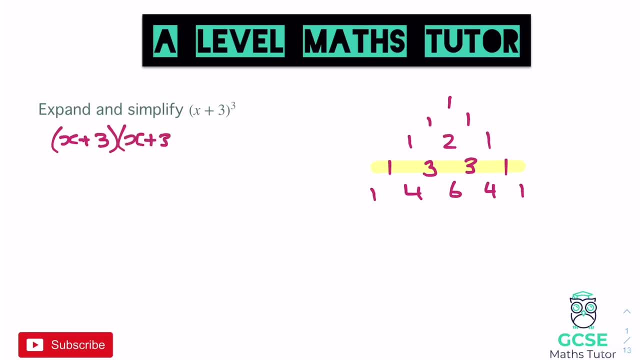 We're going to do it nice and quick though- And x plus 3. We would expand that which gives us x squared plus 6x plus 9. And then we expand that by another x plus 3.. There we go, And 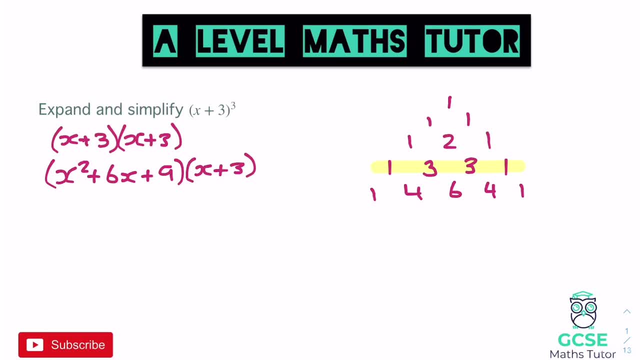 we do that and we expand this all out. We get the x squared times x gives us x cubed. The x squared times the 3 gives us 3x squared. And then we go on to the 6x and we just keep. 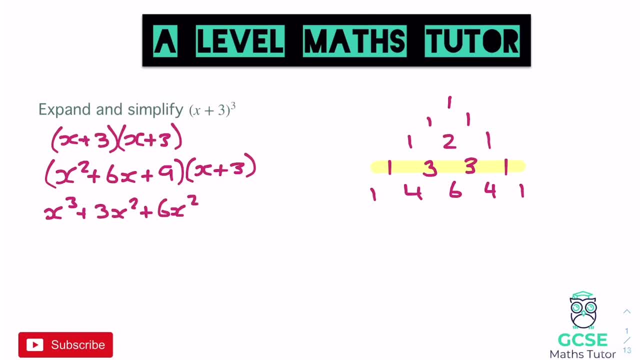 following this process. So 6x times x is 6x, squared, The 6x times the 3 is 18x, 9 times x is 9x And 9 times 3 is 27.. Okay, and we simplify this all down, so eventually we get x cubed plus and we've got those two. 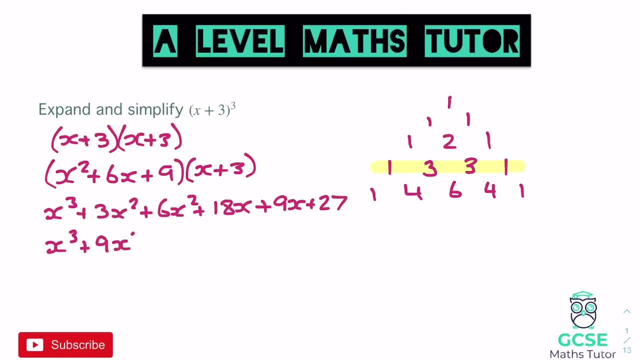 lots of the x squared there, which gives us 9x, squared The 18x, and the 9x gives us 27x. There we go Plus the 27. And we end up with these 4 pieces here And, as you can see in 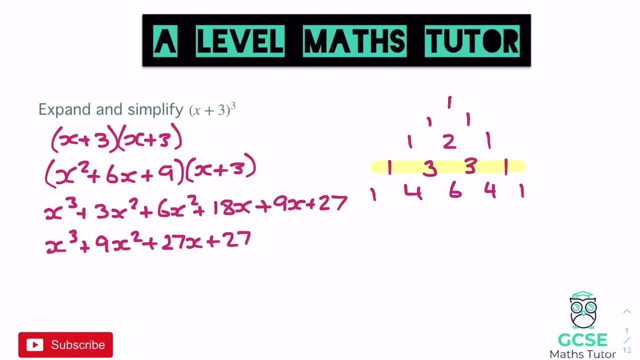 that line we've got those 4 pieces here. And, as you can see in that line we've got those 4 pieces here. Now it's not quite as clear with the triple bracket here or with the bracket to the power of 3 as to where we have those two lots of 3 in the middle, but essentially we kind of 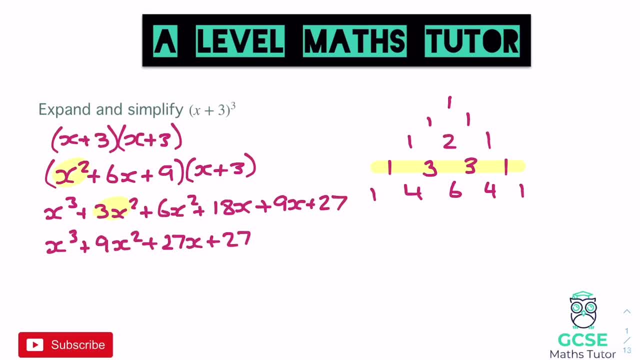 got. and lets have a look. we've got the x squared here, 1,, 2,, 3 pieces of x squared, and We've also got 3 pieces of x. We've got the 18x, the 9x, the 6x and then obviously, 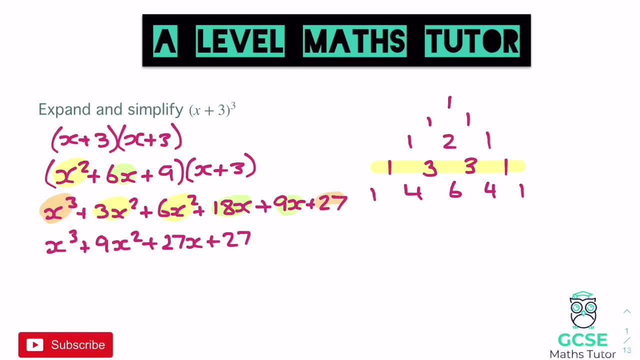 we've got the numbers on either end of here as well. We got the x cubed and 27.. You can- kind of we can- see where this pattern comes from. You've got the one lot of the x cubed, one lot of the numbers over here and one lot of the整ites. Let me go back and search. 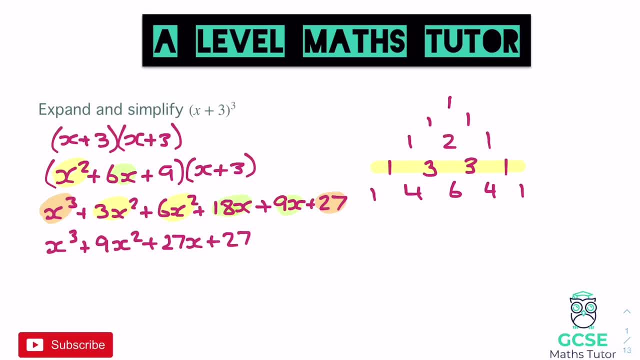 number at the end and then the three of each piece coming in the middle there, Obviously, eventually we got 2x cubed plus 9x squared, plus 27x plus 27. but we're going to have a look at how we can actually get to that using binomial expansion and using this process within Pascal's. 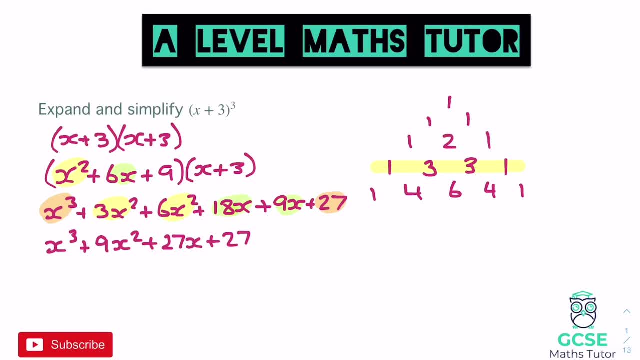 triangle. Now, obviously we don't want to have to always draw this triangle out every time and thankfully there's a nice little button that we can use to get that. on the calculator- and if you have your calculator, this is a calculator topic- it's a button that looks like this and it tends 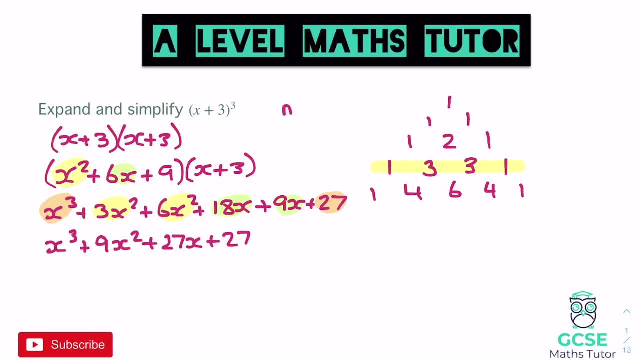 to be that you've got to press shift to get there first, but it says ncr. It's normally behind the divide button, so you normally have to press shift, divide, and it gives you this ncr. Now, in order to get these numbers here, which was what we're going to use for the first one, we have to press 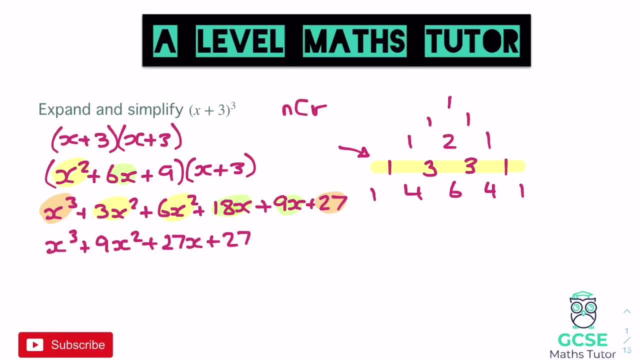 obviously it's a power of three. so we press three, shift that ncr button and you'll get a c, and then we press zero for the first one, so 3c0, and that always gives us a value of one. We always get that one for the first one, which is just there. Now for the next one, we press three. 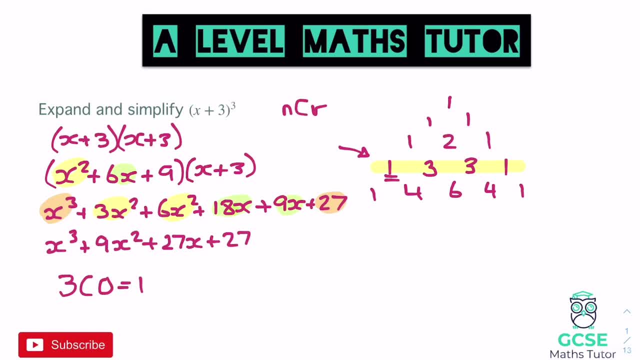 again 3c1, and we get 3c1 and that gives us three. Then we do it again, so swap the one, but I'll go for two this time. so 3c2 and that gives us. let's just have a look- we get three again. 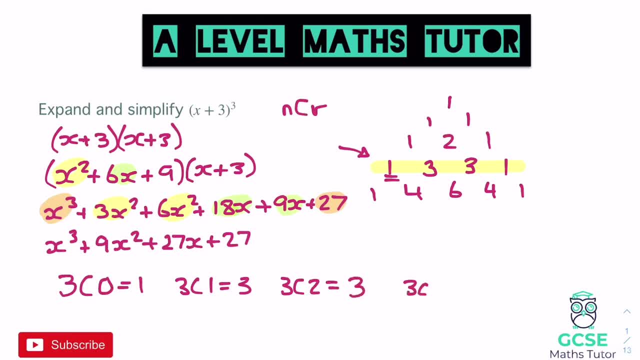 and then for the last one, we're going to do 3c3, which gives us one. So make sure you know what button is in your calculator. It's normally just behind the divide. so three, shift, ncr, and then whatever number we're looking for. We start with zero, and then one, two, three for those next ones. 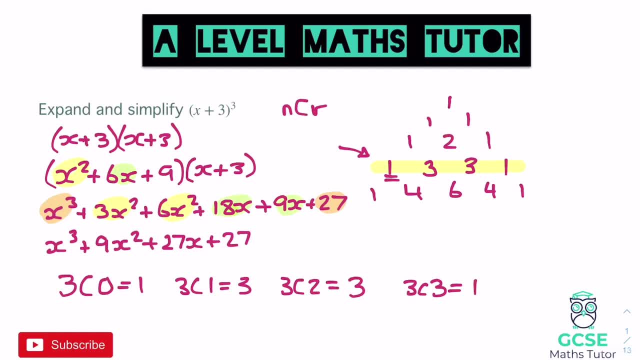 So we can actually find out what the pattern is going to be, just using this button on our calculator. I'm going to be using that throughout the video, so this is going to be a very important little button. I'm going to be using that every question and I'm mentioning that as we go, but as 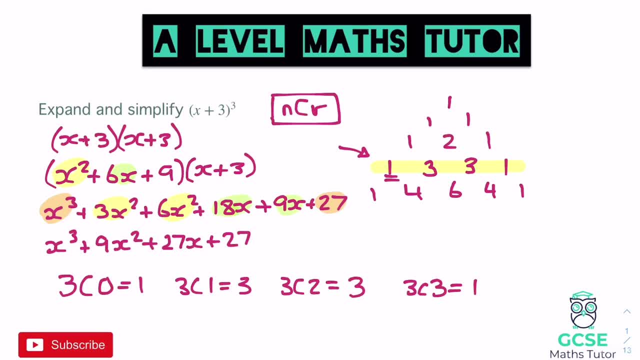 I said you've got to press shift first to get there. So let's have a look at how we can actually use that on this question, making sure that we can obviously expand this triple bracket using binomial expansion before we do that. So let's have a look at how we can actually use that on this. 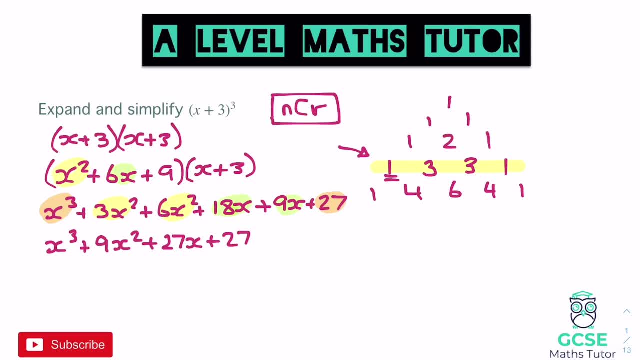 so if we get rid of this, obviously we can get rid of all of this. We know what answer we're trying to get to, and that's this one here: x cubed plus 9x squared plus 27x plus 27.. Okay, so we obviously 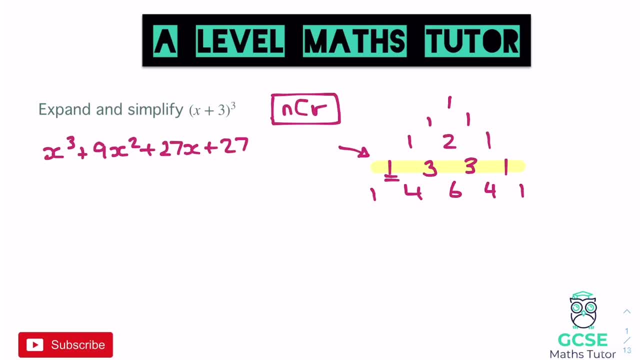 know that from GCSE level that that's going to be the answer, and let's look at using binomial expansion to get there. So, once we've got the pattern, then, and we've got, nc0 is one, and we've got one, three, three and one, and that's going to be our pattern. Now what we do is we look at the 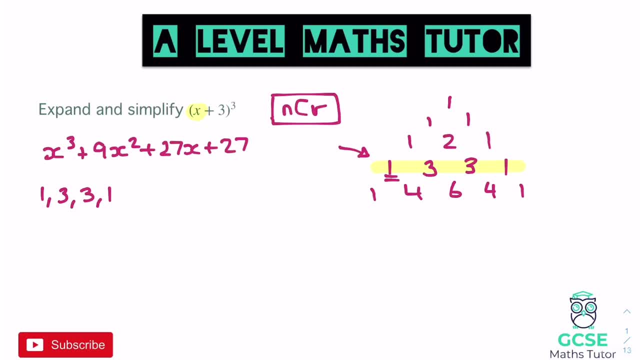 two pieces within our bracket. So we've got one, three, three and one, and that's going to be our pattern. So we have an x as the first one and a three as the second one. Okay, and let's just actually just highlight that in different colours We've got an x and we have a three. So that first. 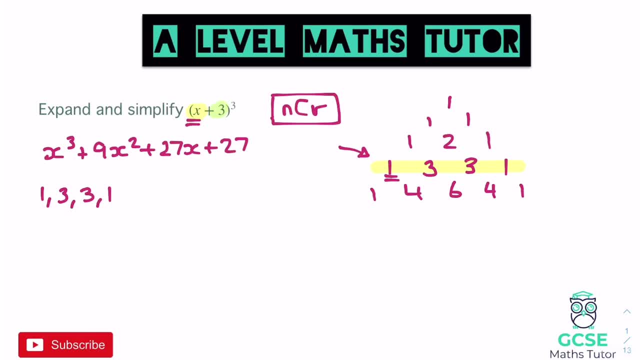 piece, and that one there, the x, is obviously the first piece in our pattern and we have one of those. So we have one lot of and that's going to be x, and everything here is going to have to be up to a power of three, So that's going to be x to the power of three and we have one of those. 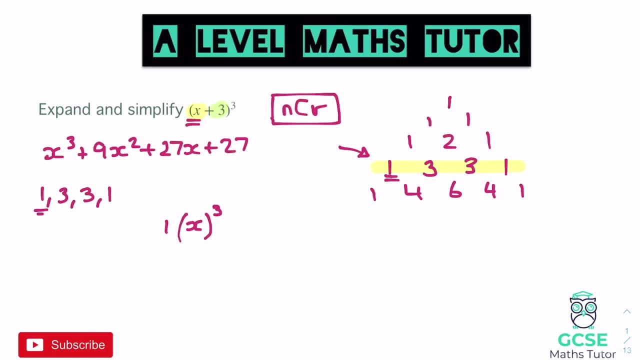 So all of these little pieces we're going to write now, we need to make sure there's always a power of three in all of them. Now the next one. we're going to have three lots of this next piece, So we're going to add to that. 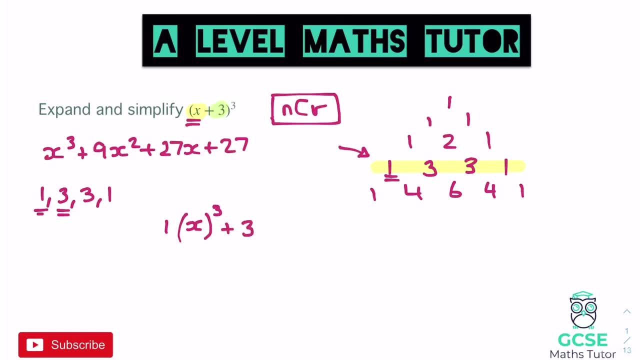 three, lots of, and the next piece is ever so slightly different. Now, x, the first one. we're going to drop down that power now because we only have one of those x cubes in there. So that x piece is now going to go down to a power of two. So one x to the power of two, But we need to make sure we 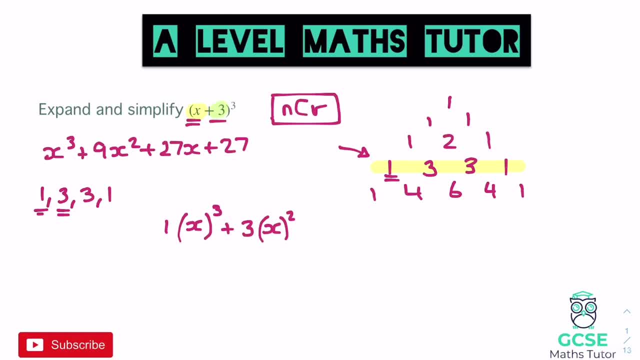 balance out these powers, and the next piece that we're going to throw in there is that three. So we have then a three, and that's going to be to the power of one, Not that we need to write the power of one there, Okay, so 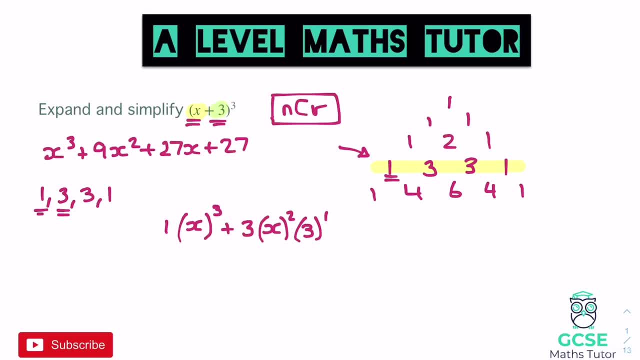 all we're going to do is reduce that first piece, which in this case is x, So that's gone down to a power of two- and introduce that next piece in the bracket, which is a three, And we're just going to swap these around now. So the x is going to keep reducing and that number, the three, is going to. 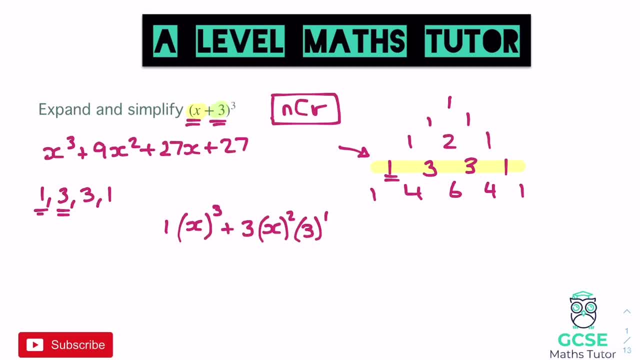 keep going up in powers until we get to a power of three for that one as well. So the next one, and again we've got three lots of this next piece. So we're going to add to that three lots of- and we have x- to the power of one. this time That's going down to the power of one and that three is going. 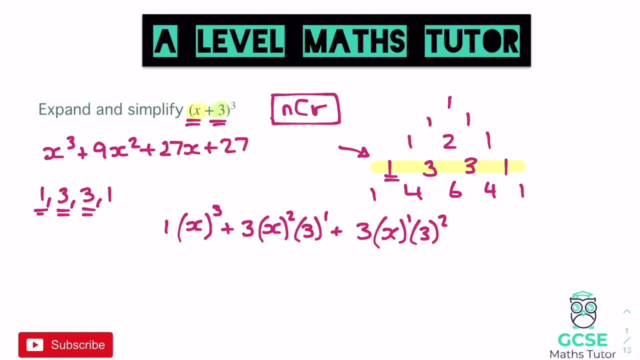 to go up to a power of two. There we go, And that's our third piece in that pattern done, And then on to the last piece. we have one of these, So we're going to add to this one of Now. x is going to go down to the power of. 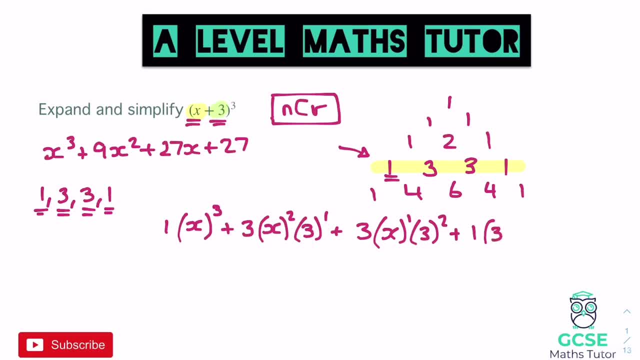 zero. So that's gone and we just have this three at the end, which again has to balance out to that power of three. So one lot of three cubed And if we expand these all out and see what we get, One lot of x. 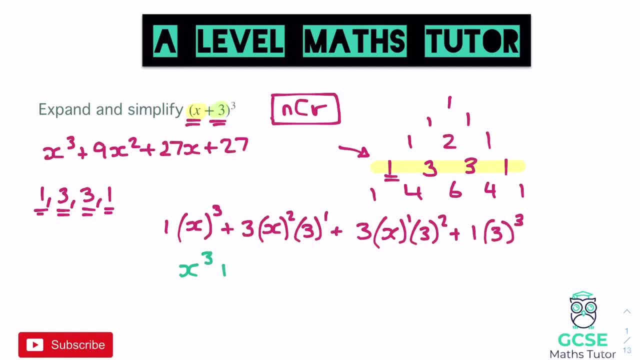 cubed is x cubed. There we go. Then we're going to have three lots of x squared times three. Well, let's just do the three times times the three to start with, which is nine. So that's nine lots of, and then we've got x squared. 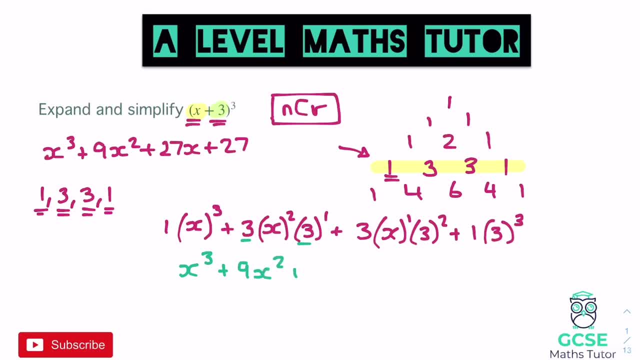 with that, so nine lots of x squared. Then for the next piece, let's have a look. We've got three lots of three squared. Three squared is nine, Three times three squared. so three times nine is 27.. Again with that, x to the power of one, so plus 27x, And then at the end there we have one lot of. 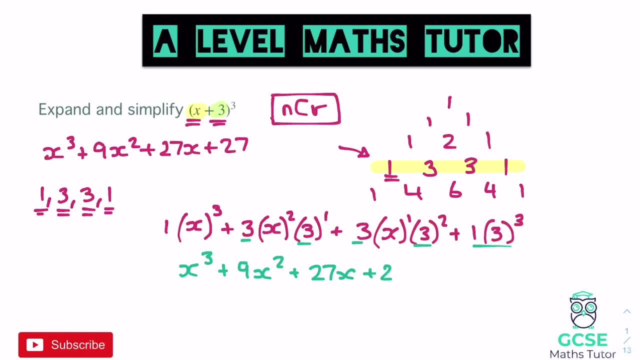 three cubed. Three cubed is 27,. so plus 27 at the end. And there we go. That matches obviously what we've got from expanding our triple bracket. at the top We've got x cubed plus nine, x squared plus 27x plus 27.. So that's all we're going to do for binomial expansion. Obviously it gets a little. 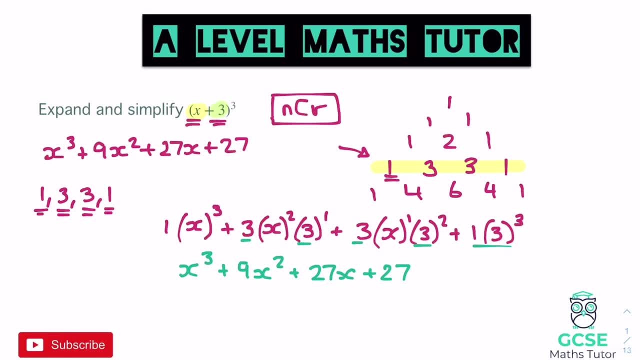 bit more complicated as we start to go further down Pascal's triangle and start to get larger numbers involved. but basically that's all we're going to do. We're just going to write down what the numbers are in, obviously, in that line of Pascal's triangle that we're going to be looking. 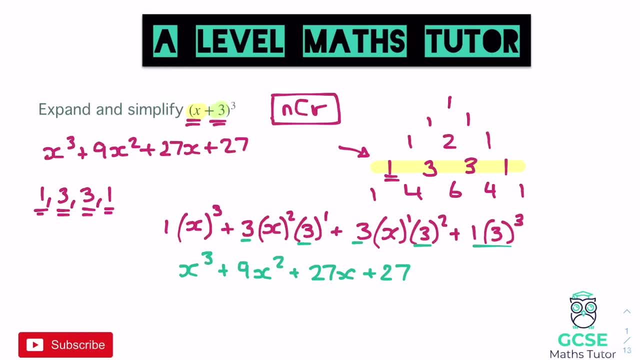 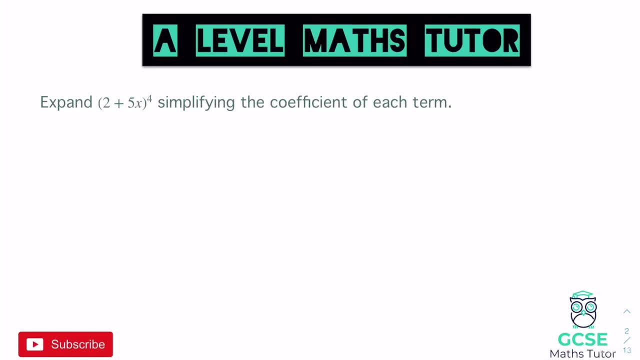 at, and obviously just balancing that out with our powers, sort of moving through. But let's have a look at another one and see how we can apply this to a slightly harder question. Okay, so we have expand two plus five x squared x, to the power of four, simplifying the coefficient of each term. So let's have a look at this one. 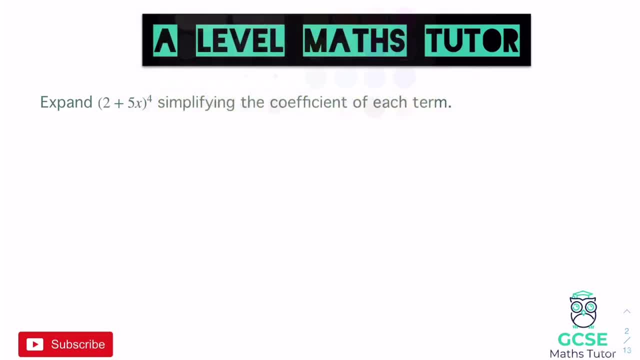 then Now, in this particular question, we've got a power of four. So for a power of four, we're going to first find out what the pattern is of Pascal's triangle. at that point I'm going to use the calculator to do this. So we're going to do four, c zero. So I'm going to do that on my calculator. 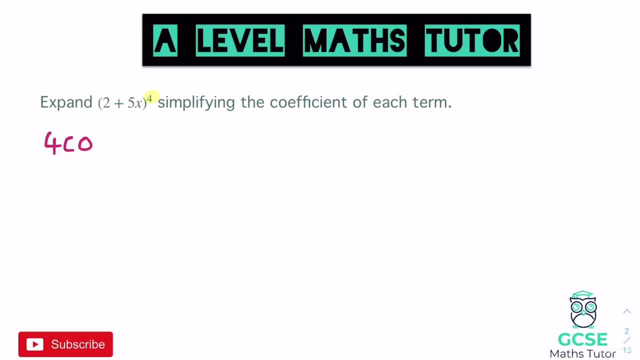 now Four shift ncr button zero and we get one. So we've got one for the first one. Swap the zero is four, Back in, swap it for a two, So four c two is six. Back in four c three, which is four. 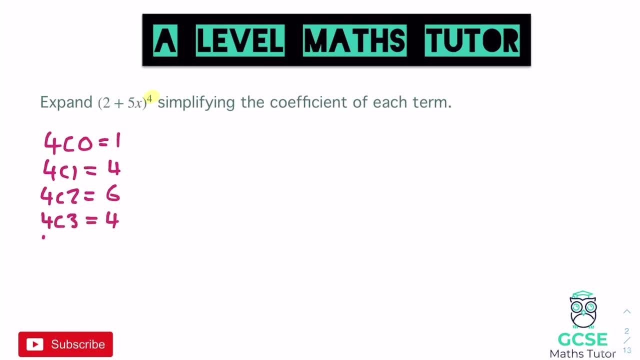 And then four, c four, which is one That gives us that line of the triangle there. Now, having a look again, we know it's a power of four, so everything's going to have powers of four. in this one We've got our first piece, which is a two, and our second piece within the bracket, which is a positive five. 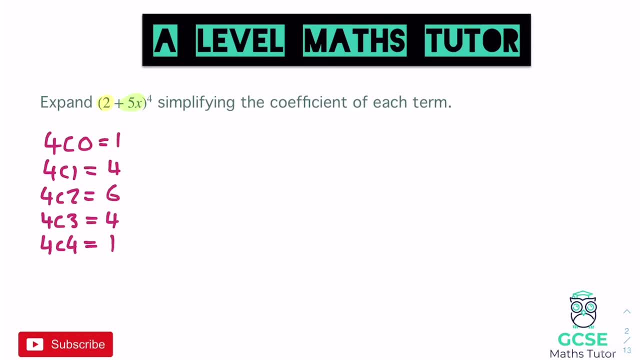 So if we start writing this down, well, we've got one to start with, Let's start with the one. So we've got one lot of the two, the first piece and that's to the power of four. So one lot of the two. 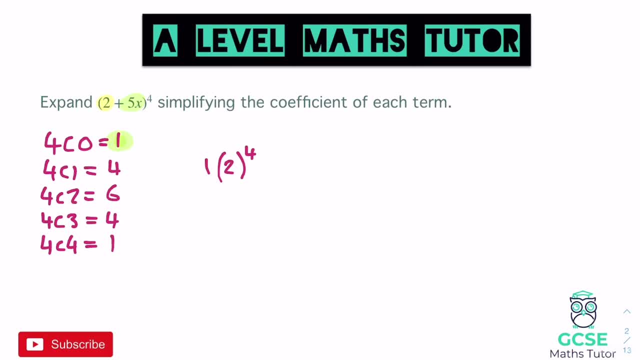 to the power of four. Just like with all normal double and triple brackets, we always get that first piece there at the start to the power of four. On to the next piece, We get four lots of this next one. So we've got four lots now. So we're going to add to that four lots of and we've got. 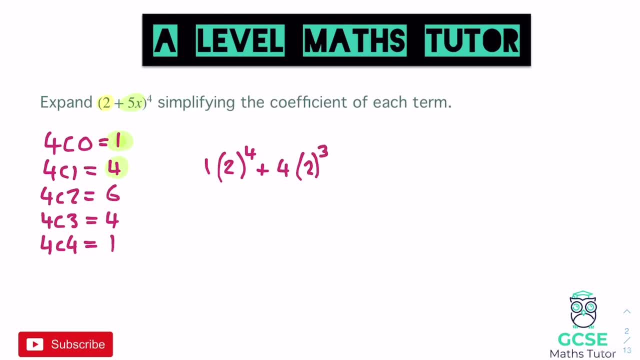 two which is now reduced to four. So we've got four lots of, and we've got two, which is now reduced to a power of three, And now introducing that next piece which is the five x, So one lot of the. 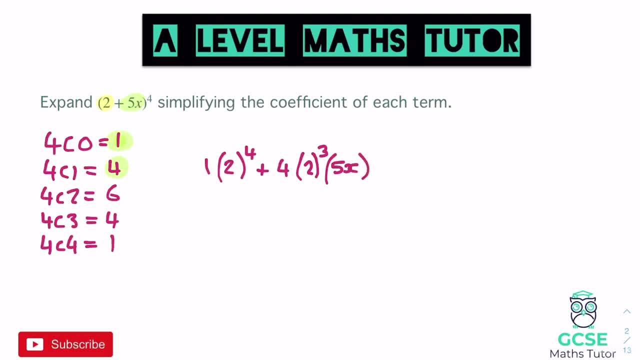 five x. I won't write the power of one this time, but we've got one lot of that. Then we've got on our next line, we've got six lots of this next one. So we have six lots of, six lots of, and we've 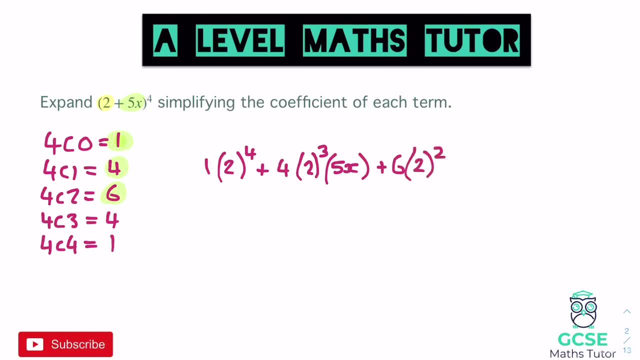 got two being reduced to a squared and five x increasing to a power of two. There we go, And on to our next one. Let's have a look, We've got four. lots of this one as well. I'm going to run. 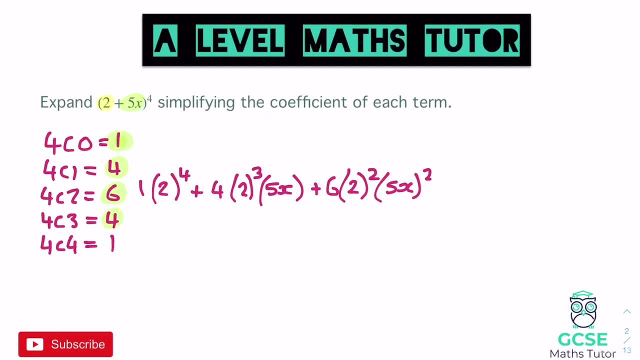 out of space here. Let's move on to the next one. So we've got four lots of this one as well. Let's move this to the left a bit. There we go. So we're going to have four lots of this next one. 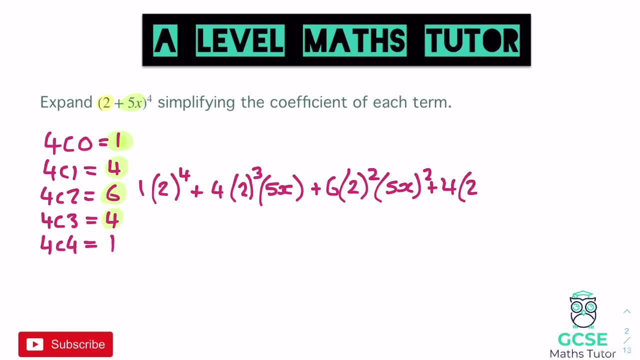 So we have four, lots of two, which is now down to a power of one- It's decreased- And the five x, which goes up to a power of three. And there we go, And now on to our last one, And we have one. 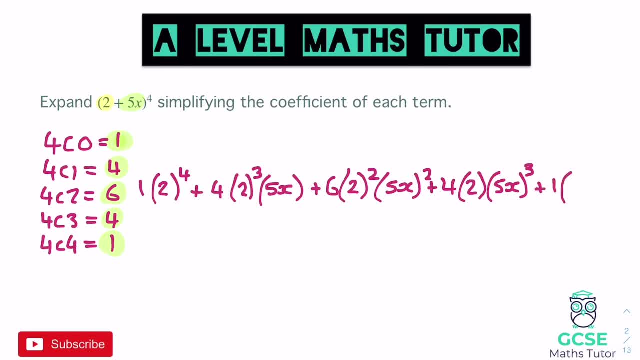 of these. So we have one lot of, and it's five x this time to the power of four. There we go And notice: on every single piece there we've got a power of four, Even though I've not written in. 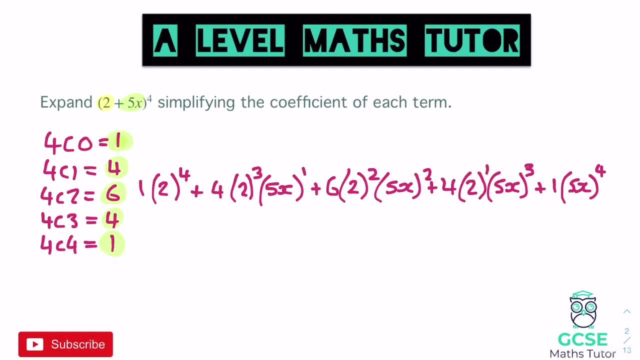 these ones. I could write a power of four. I could write a power of four. I could write a power of three. I could write them in. If you have a look, both pieces there. In total, we've got a power of. 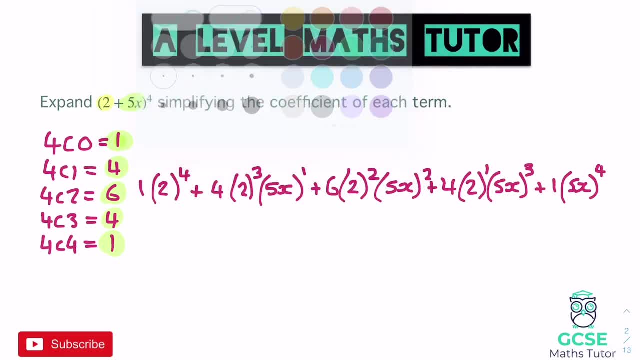 four on every single piece. Now, if we go back expanding all this and simplifying it down, let's see what we get. And again we're using a calculator here. So we've got two to the power of four is our first one, which is 16.. So 16.. Then we have four, lots of two cubed. Let's have a. 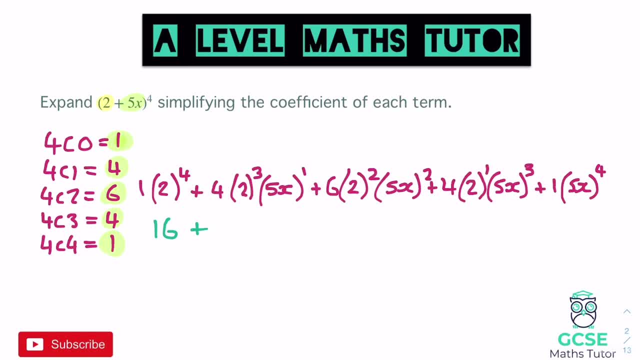 think So. two cubed is eight times that by four is 32.. So we've got 32 lots of five x, which we'll sort out in a sec. Then we have six lots of two squared. Two squared is four, So six times four, which is 24.. So we have 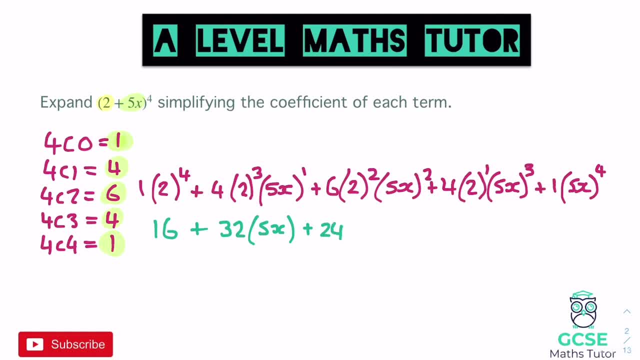 24 lots of and five x in brackets. squared is 25 x squared. There we go. It's just squaring both of those Again. you can use your calculator for that. For the next bit, we've got four lots of two. So 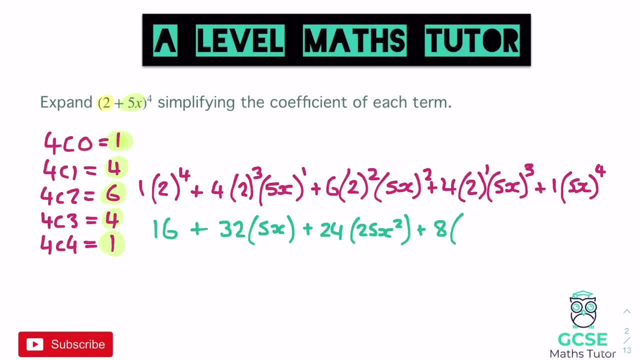 that's eight lots of. and then we've got five x cubed in the bracket which is 125 x cubed, And then, for the last piece, we've got four lots of two. So that's eight lots of. and then we've got. 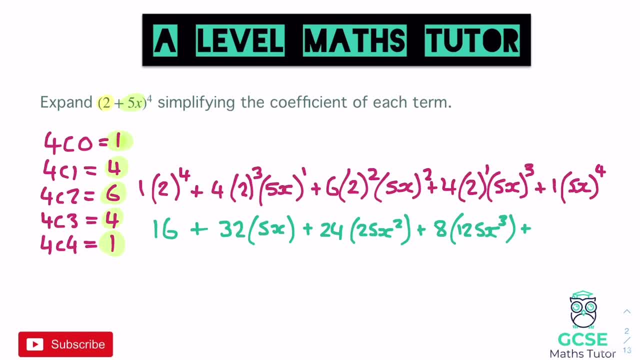 five x to the power of four. Five to the power of four is 625.. So we have plus 625 x to the power of four. There we go. Last little bit of sorting out to do, because we've got a couple there that we 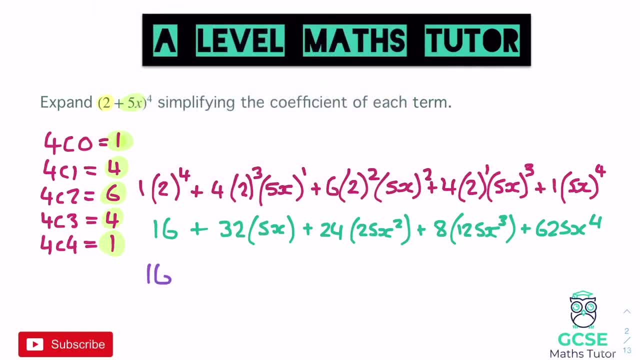 can simplify a bit more. We've got 16 at the start, which is fully simplified: 32 times five x well, 32 times five is 160.. So we get 160 x 24 times 25 for the next one, which is 600.. 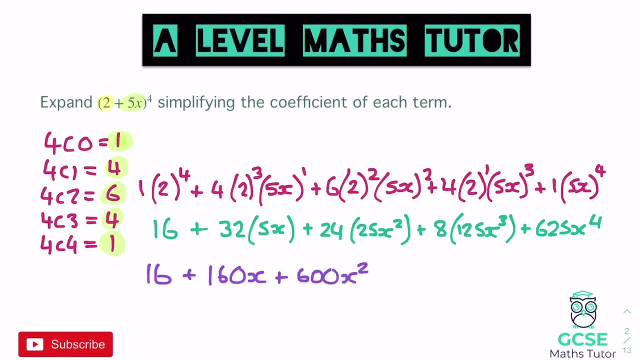 So we get 600 x squared Eight times 125 for the next one, which is 1,000.. So we get plus 1,000 x cubed, And then plus the 625 x to the power of four at the end. there, There we go, And that finishes. 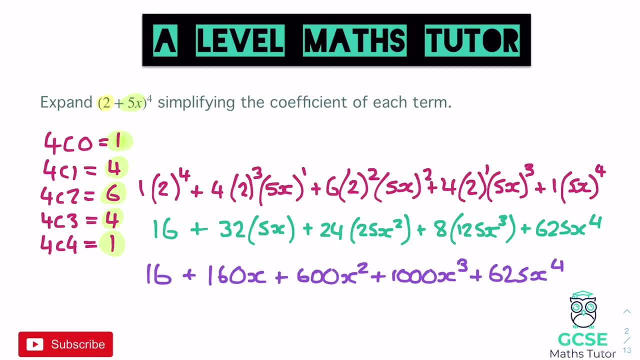 that off. So obviously, as you can see, it gets a lot more complicated when we've got these higher powers And it's harder to see the pattern than it is to see it with a double bracket, where we have a bracket squared, Because obviously the actual process for expansion is going to be a lot. 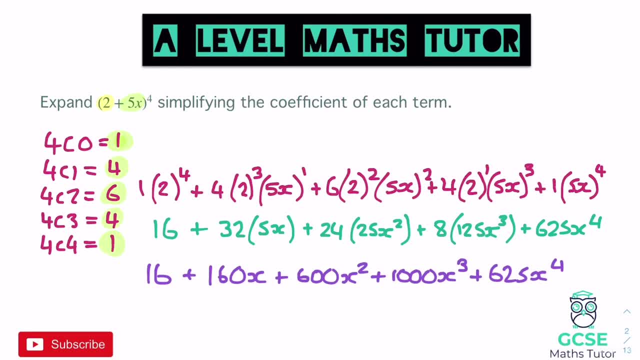 more complicated. So expanding all this would be very complicated. Obviously, we'd expand two brackets, times it by another, times it by another, And we'd get so many of these pieces that it would just take absolutely ages for us to expand. So here's a nice quick way of us expanding these. 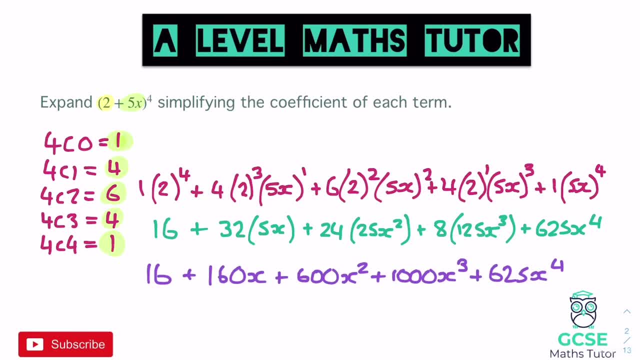 and following those patterns. Okay, but it's all about, obviously, when we've got these two pieces. the first piece, which I've got highlighted in yellow up here, starts off with that power of four and just decreases in power until it disappears, And that piece on the right there 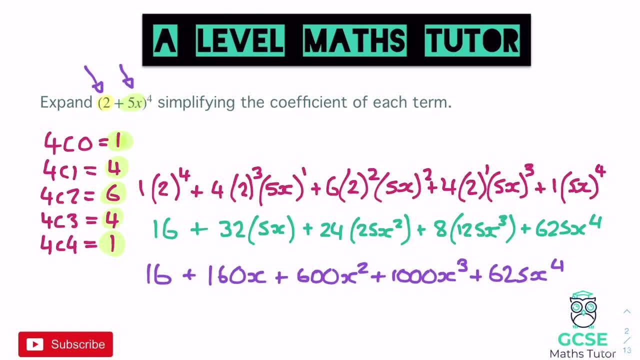 obviously is introduced in the second piece and starts increasing in powers right up to the end where it finishes on that final power of four. We're going to have a look at another one of these before you have a go, So let's have a look at that. 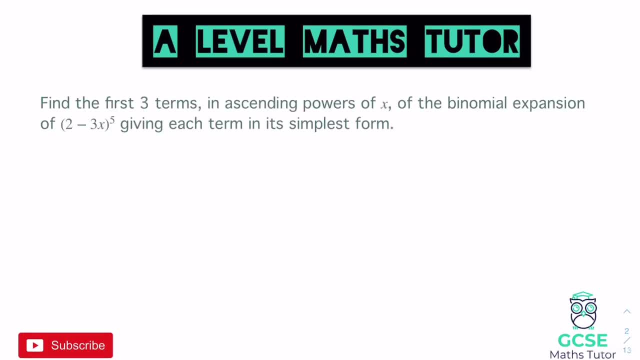 one. Okay. so there's some slightly different language in this one It just says: find the first three terms, And that's because it's starting to get up to the power of five. And as you get to the power of five or six, seven, eight, nine, ten and beyond, there's so many pieces to write down. 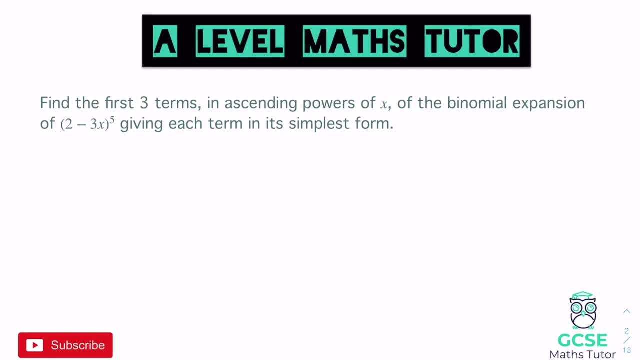 it just takes absolutely ages to write them. So we tend to just be asked for the first three or the first four terms And it says in its ascending powers: of x, here obviously just writing it as we have done to start with. So this is off: the binomial expansion of two minus three x to the 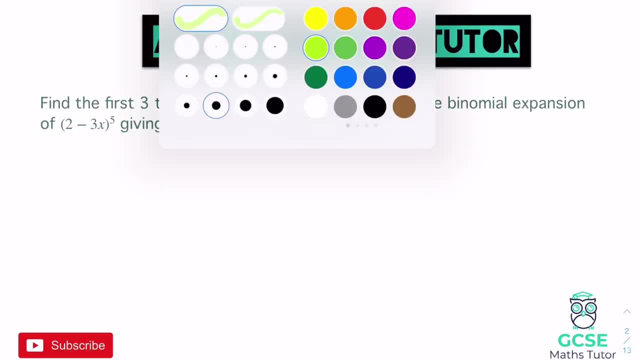 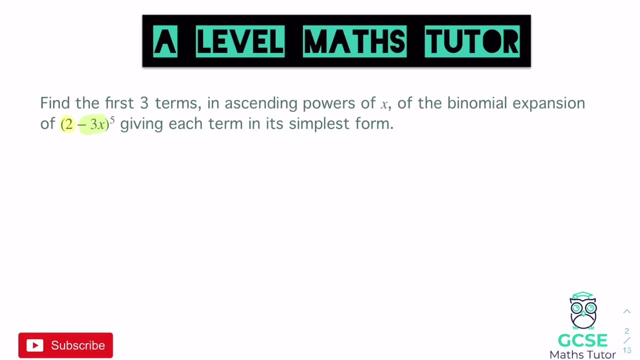 power of five, And again given each term in its simplest form. So if we have a look, obviously, in this one here, our first piece is a two And our second piece this time is a negative three x. We're just going to have to watch out for that negative on this one, But that shouldn't be any. 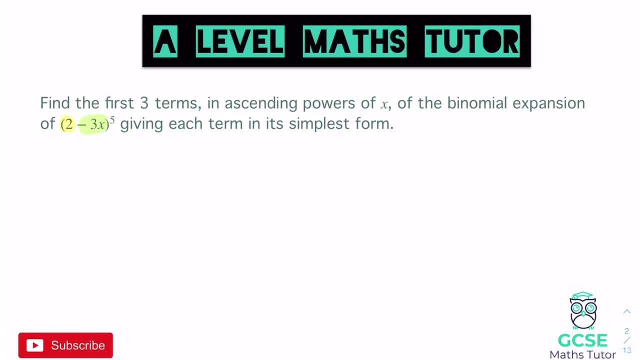 problem really, as we're using a calculator as well. But obviously we just need to find what the first three parts of that pattern are. So for the first three terms, when we have a power of five, So easy enough to do on a calculator, we do five c, zero, which is obviously one, always for. 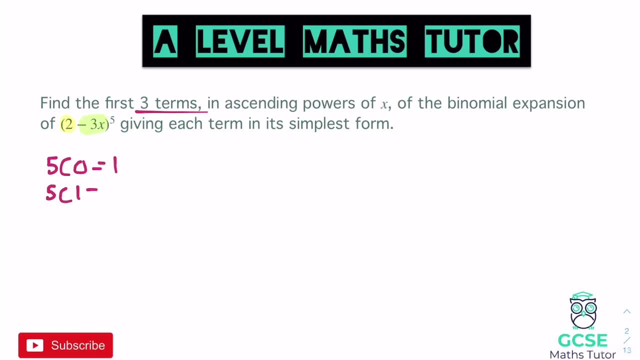 the first one. Then we're going to do five c one, work that out, And five c two. That's going to give us our first three patterns of Pascal's triangle on that row. So let's have a look: Five, And we have c one, which is five. There we go And swap that for a. 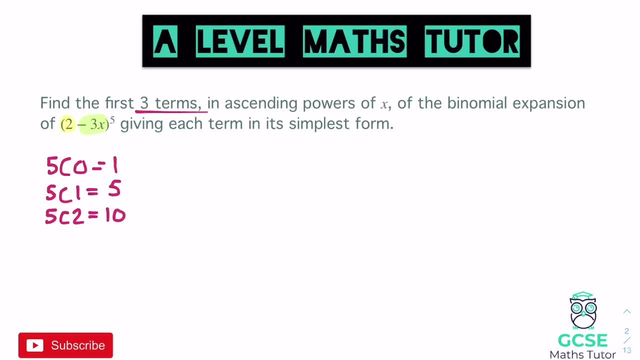 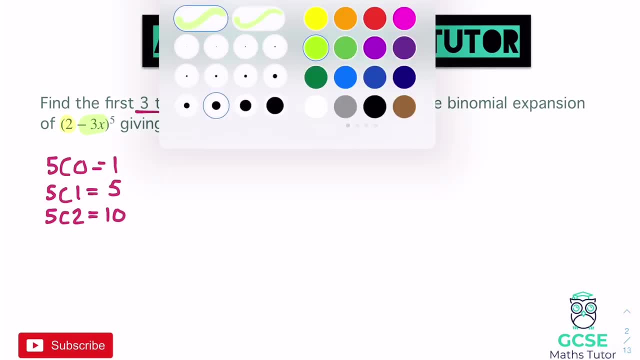 two, So five c two, which is ten. There we go. So there's our first three pieces, or the first, the amount of each piece that we're going to have in this expansion, Right? So let's have a look. So the first one: we have one lot of. So we have one lot of. 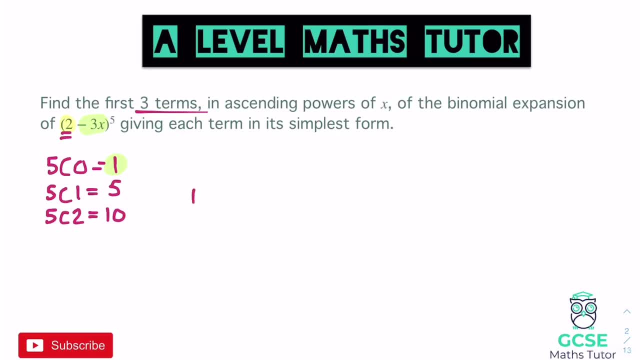 And that piece, there is a two, the first piece. So one lot of two, And again, make sure we have that power of five in there. And then for the next one, let's have a look, We're going to have five lots of. So we have five lots of And we've got the two, which is reducing now to a power of. 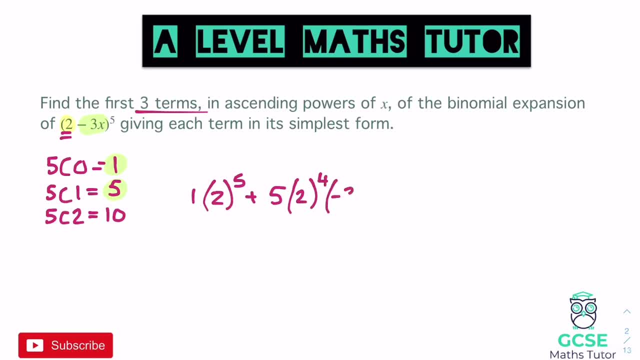 four, and introducing that negative three x, I'm going to keep everything in a bracket just to make sure I don't mess up with these symbols in front of it at any point. So negative three x. There we go, And for the next piece, we're going to add to that. 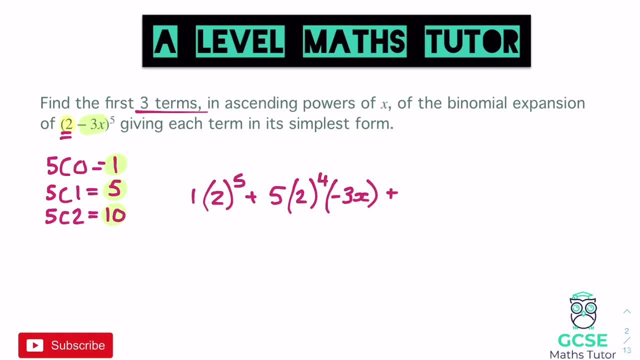 And again, have a look here. We've got ten lots of this one, So we have ten lots of, And it's two being reduced to a power of three, And that negative three, x is going up to a power of two. There we go, And there's our first three, And obviously this continues, but we are already finding the first three here. 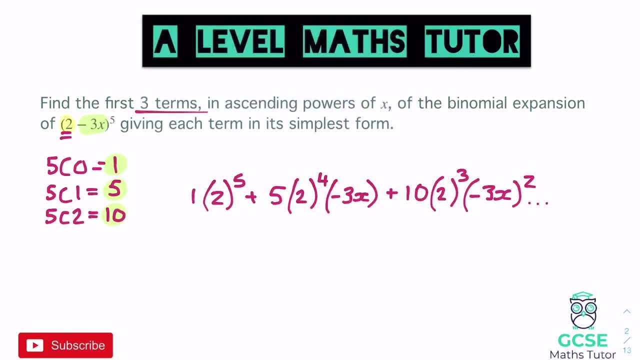 So let's simplify this down. See what we've got. So one lot of two to the power of five, or two to the power of five, on the calculator is thirty two. There we go, And we're going to add to that. Let's work that out to start with. five lots of two to the power of four is eighty. 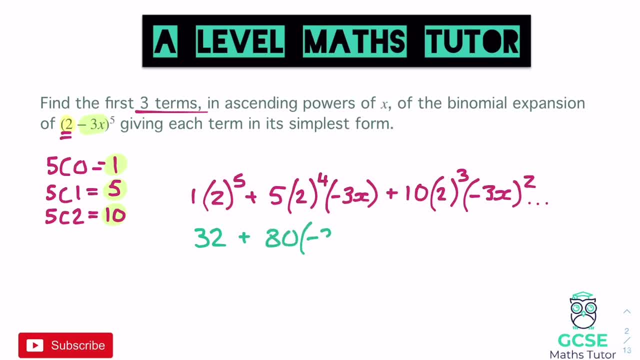 So we're going to add to that eighty lots of negative three x, which is going to be a negative piece, And we'll deal with that in a sec. And I'm going to add to that to ten lots of two cubed, which is eighty lots of. 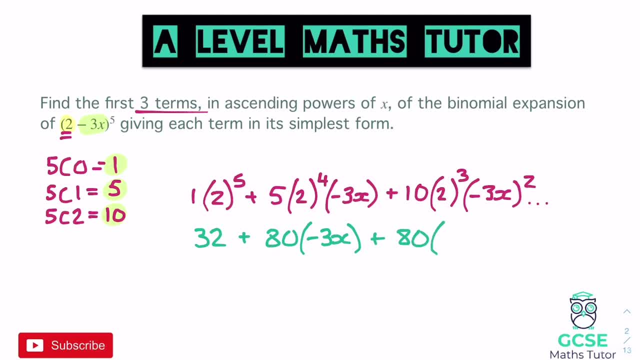 And then we have negative three x squared, or negative three squared is positive nine x squared. There we go, So we have positive nine x squared And obviously just then simplifying this down, So we've got thirty two to start with, And we're going to add to that. 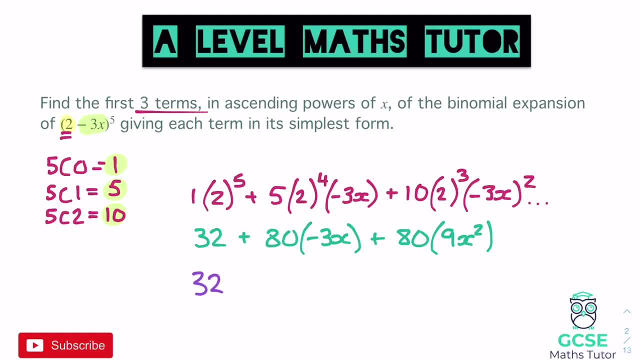 Eighty, lots of negative three x. Well, three times eighty is two hundred and forty and it's negative. So we're going to be taking away two hundred and forty x, And then we're going to add to that nine times eighty, which is seven hundred and twenty. 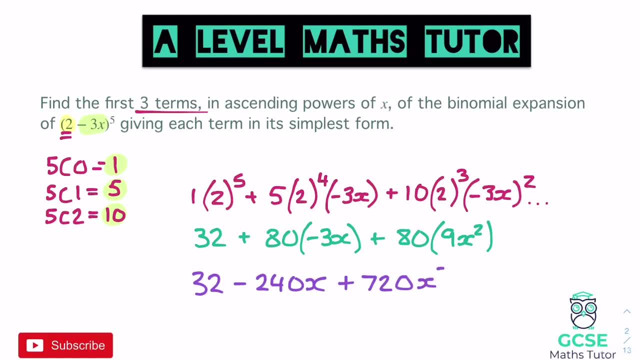 So seven hundred and twenty x squared, And there we go. There's our final answer, The first three terms of that expansion. there, Obviously, we could continue. We could keep doing Pascal's triangle there: Five lots of the x one, then one lot of the final one, and keep on going. 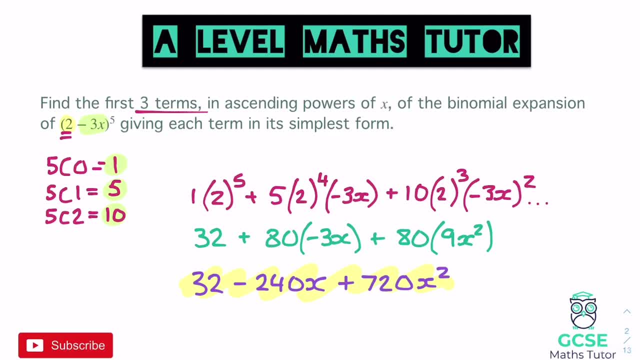 It only asks for the first three. It's easy enough there. We only have to do those first few. So obviously this is really important here And knowing to use this button. obviously five c, zero. So power of five, finding that first one which is zero. 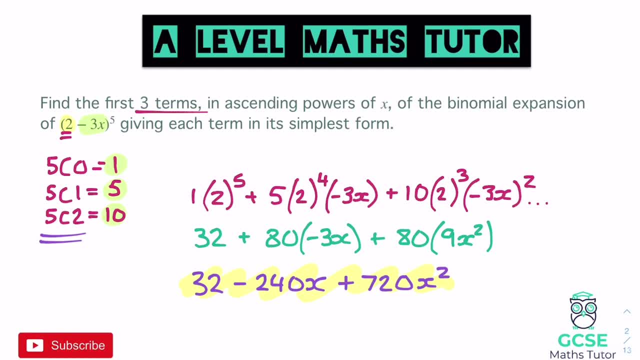 And then keeping on going with that, just depending on what the power is there. Obviously, if you said power of seven, we would do seven c zero, seven c one, seven c two And just incorporate those numbers in front of the coefficients. there, just to make sure that we simplify it all down correctly. 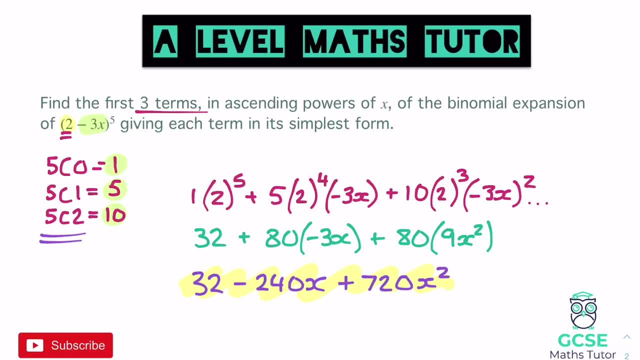 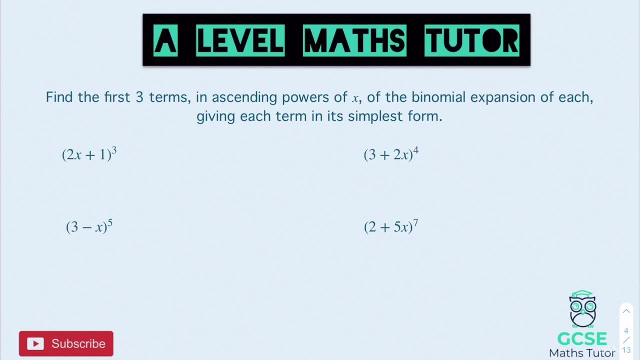 But there we go. That is how to go about doing these. first, lots of binomial expansion. So here's a couple of questions for you to have a go at. OK, so here's four questions. so pause the video there, Have a go at these and we'll go over the answers in a sec. 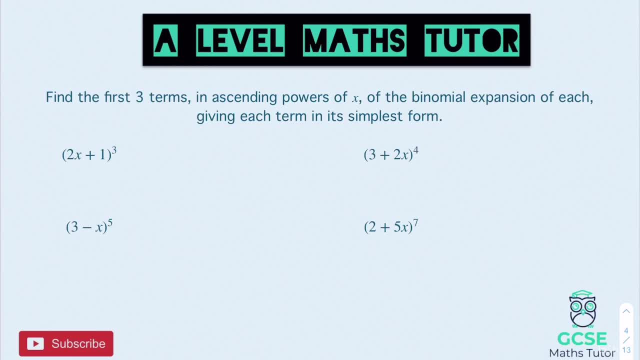 OK, so for the first one. Now, obviously this is only a triple bracket here, so this is obviously one that you could do without using binomial expansion, but quite a nice one to be able to actually check your answer using that whole process from GCSE. 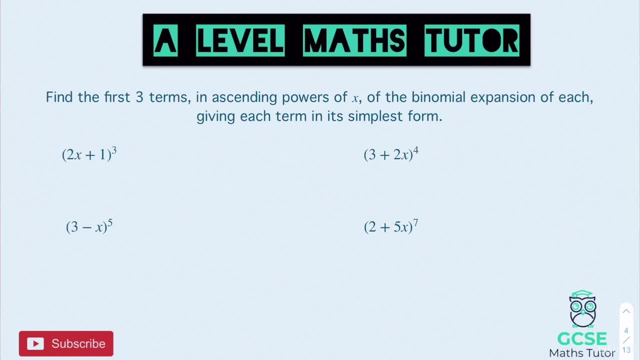 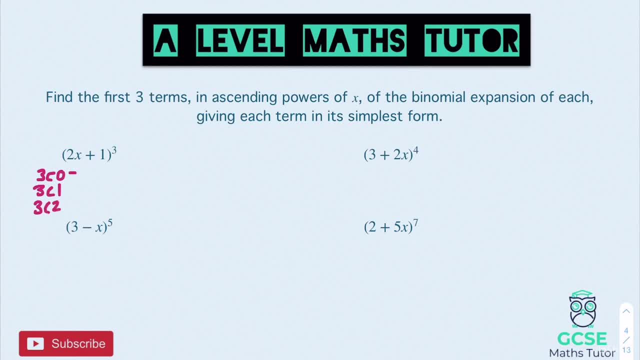 3c1 and 3c2.. We need to write down what they are. Obviously, that first one is always 1,, that's okay. Then we've got 3c1, which is 3,, and 3c2,, which is also 3.. So, in terms of expanding, 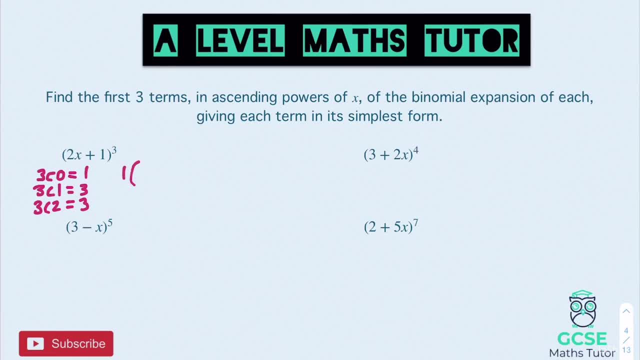 this. then we have one lot of that first piece there, which is the 2x, and I'll just highlight these. We've got the first one, which is 2x, and the second one, which is 1, there, So we have 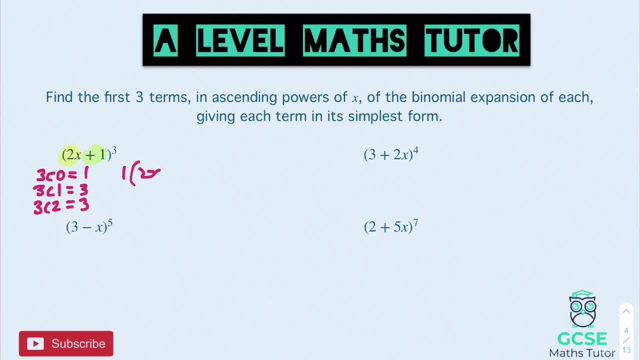 one lot of the 2x which is going to be cubed, and we're going to add to that 3 lots of the 2x which reduces to a power of 2, and then the 1, which is just a power of 1.. And then the last one. 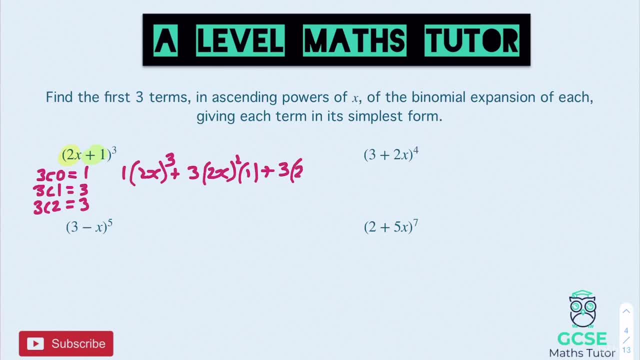 we've got 3, lots of, and we've got the 2x again, which is now a power of 1, and the 1, which is going to be squared. There we go, And if we simplify all this down, let's see what we get. 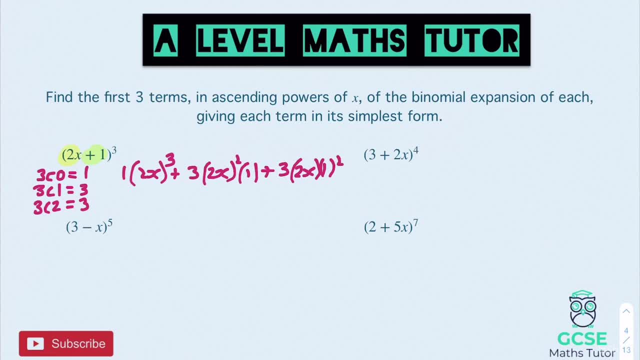 So we get one lot of 2x cubed, so 2x cubed. 2x cubed is 8x cubed. 3 lots of 1 on, the next one is 3, and that's going to be 3 lots of 2x squared, which is 4x squared. there we go. and then we get 3- lots of there's 3 times 1 there 3 lots of the 2x. we could probably just work that out straight away: 3 lots of 2x, which is 6x. there we go. 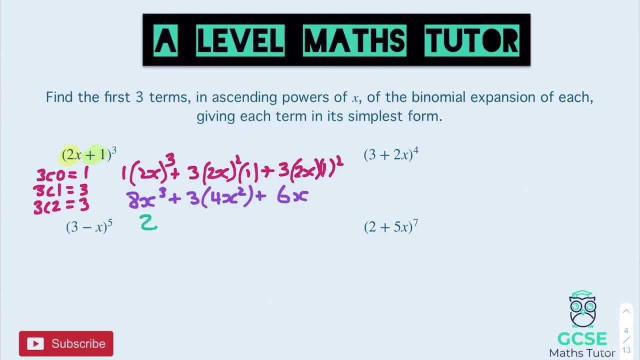 And then we just need to simplify that piece in the middle there. so we've got the 8x cubed 3. lots of 4x squared is 12x squared and then we've got the 6x at the end. there we go, and there's our first 3 times. for the first one, 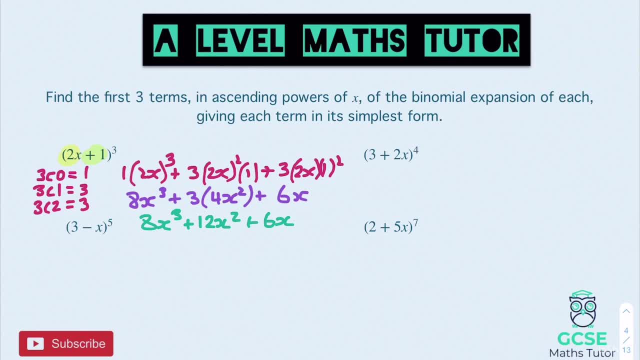 Now, obviously, let's just have a look at the one to the right of that. so we've got a power of 4 in that one. so we need to work out 4c0 to start with. so let's have a look. we've got 4c0, which is 1,. 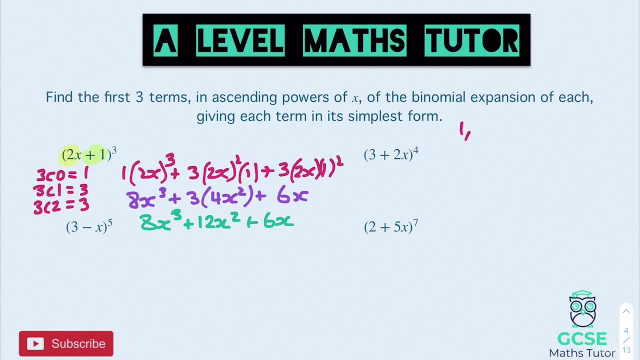 then we have 4c1,, which is 4,, and then 4c2,, which is 6,. there we go. so there's our first 3 pieces of the pattern there. so we have 1 lot of the 3,, which is. 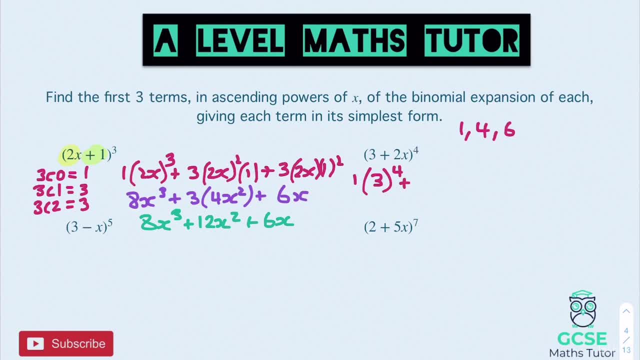 to the power of 4, then we have adding to that 4 lots of the 3, cubed this time, and then the 2x, and then for our final piece we have 6 lots of and we have 3 to the power. 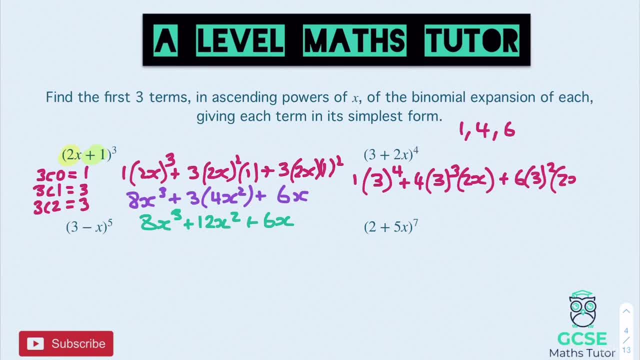 of 2, and then the 2x which is now going to be squared. there we go. so simplifying this down, let's see what we get. so 3 to the power of 4, I'm just going to do that on the calculator- is 81,. 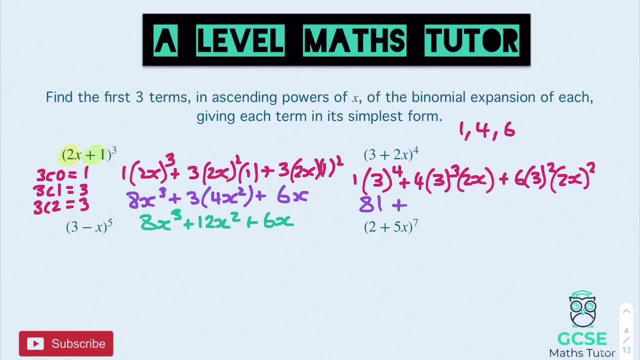 so we get 81, plus 4. lots of 3 squared, so 4 times sorry, 4. lots of 3 cubed, so 4 times 3 cubed is 108, multiplied by 2 is 216, so we have. 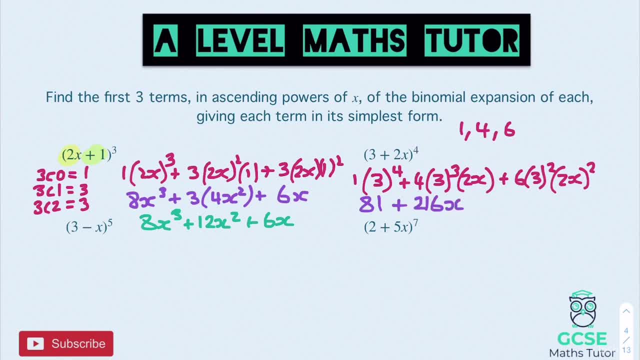 216x, and then the last one. there we've got 6 times 3 squared. so 6 times 3 squared is 54, so we're going to have 54- lots of- and then 2x squared. I'm just going to write this down over: here is 4x. 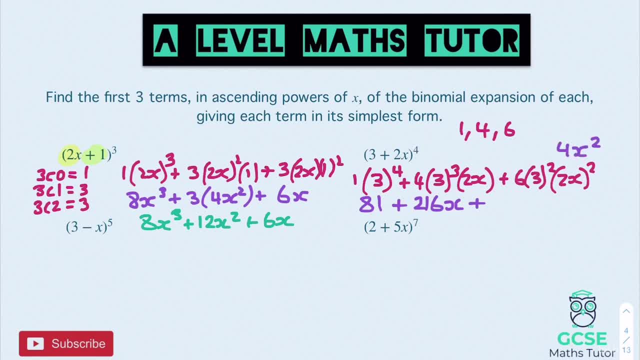 squared. there we go. so we have 54 lots of 4x squared. so 54 times 4 is 216, so we have 216x squared. there we go, and there is that one 216x squared at the end. 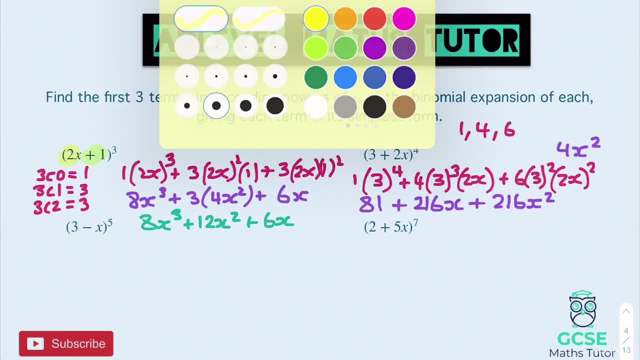 On to our next one here. let's have a look. we've got a negative getting involved here, so we've just got to be careful, because we've got 3 as our first piece and then negative x as our second piece. 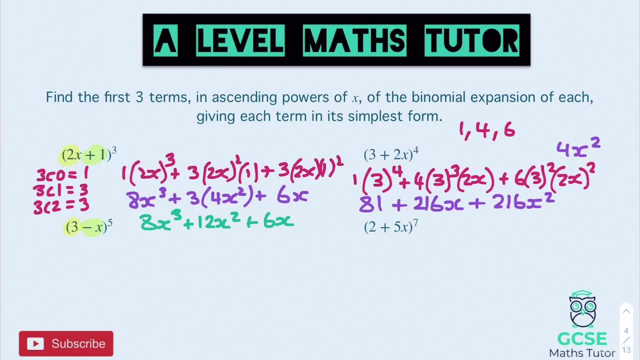 So let's just get our pattern, obviously for a power of 5,. so a power of 5, we need 5 c0,, which is always 1 to start with. so we get 1, 5c1,, which is 5,. 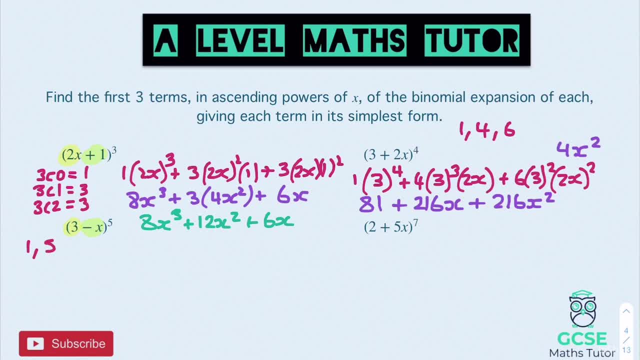 and then 5c2, which is 10,. so 1,, 5, and 10.. So let's have a look. then we have one lot of that first piece, which is 3 to the power of 5,. 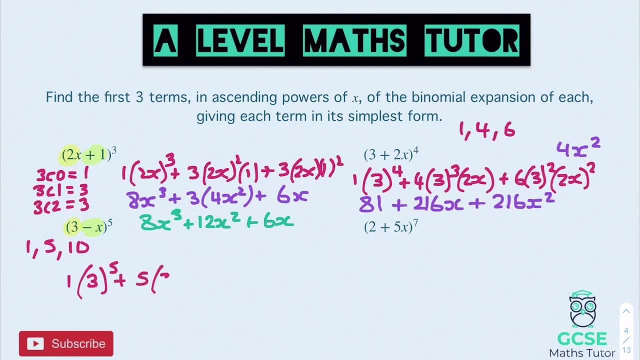 and then we're going to have 5 lots of 3 to the power of 4, and then negative x. and then for the next one we're going to have 10 lots of 3 to the power of 3, and then negative. 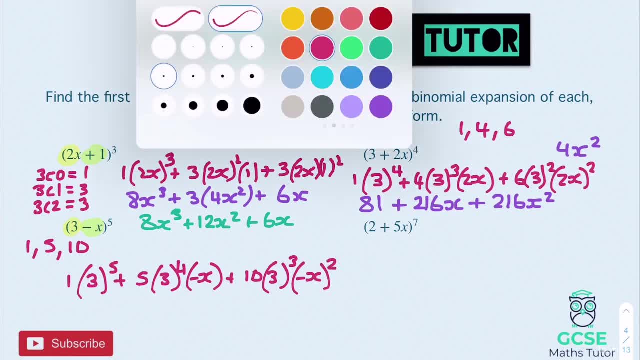 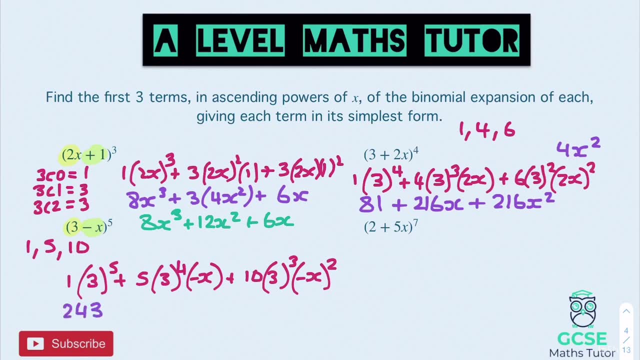 x to the power of 2.. There we go, and let's simplify all of this. so 3 to the power of 5 on the calculator is 243, so 243, then 5, lots of so 5 times 3 to the power of 4,. 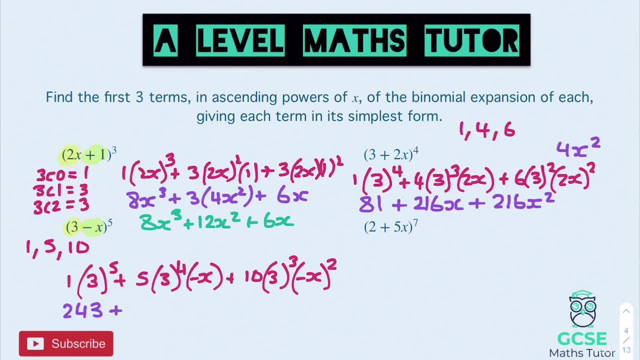 there we go is 405, but that's going to be multiplied by negative x. so we've got 405 multiplied by the negative x, which is going to be minus 405x. so let's get rid of that plus. so minus 405x. 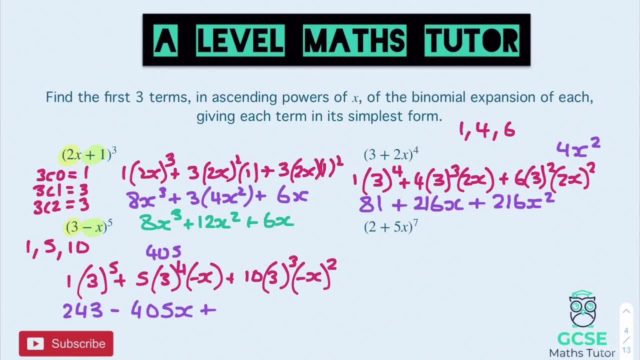 and we're going to add to that 10 times 3 cubed. 10 times 3 cubed is 270, negative x squared is going to be positive x squared, so we have plus 270 x squared. there we go and on to our last. 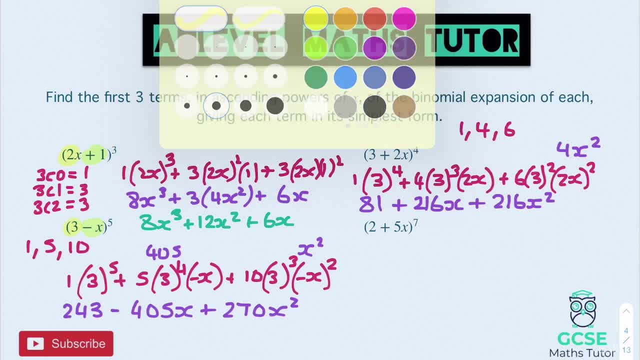 one and again, let's have a look at what pieces we have. so for our first piece there, we have 2, and the second piece in the bracket, we've got positive 5x, and this time it's to the power of 7,. 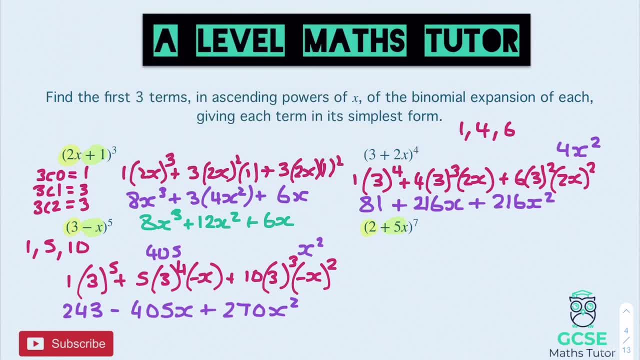 so 7 c0 is 1,, 7c1 gives us 7,, so we have 1,, then 7,, and then for the last one, 7c2 is 21.. There we go. OK, so for our pieces here. then we have: 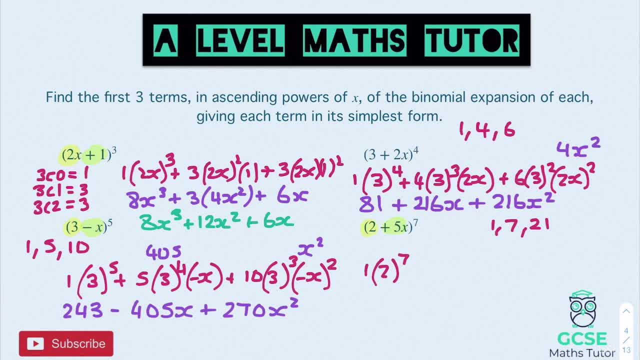 1 lot of 2 to the power of 7, and in the next piece we've got 7 lots of 2 to the power of 6,, 2 to the power of 6, and then 5x to the power of 1, and for our 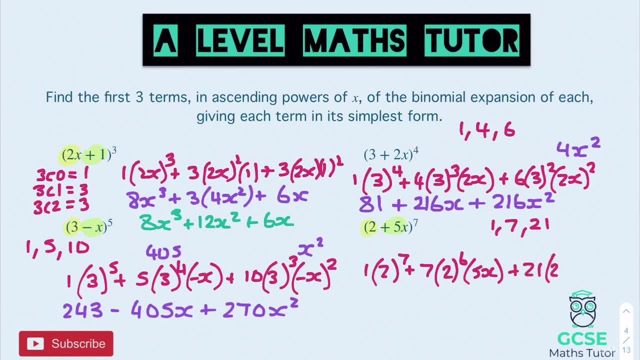 last piece, we get 21. lots of 2 to the power of 5, and then 5x squared. there we go. so simplifying this down, 2 to the power of 7 is 128, so we get 128,. 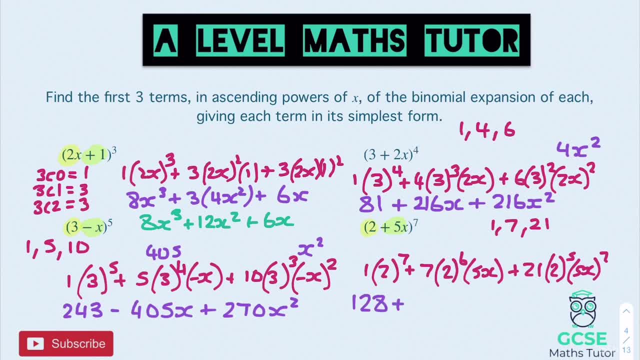 plus 7, lots of 2 to the power of 6,. well, 2 to the power of 6 just on, the calculator is 64, timesing that by 7 is 448, and timesing that by the 5 in front of the x there gives us: 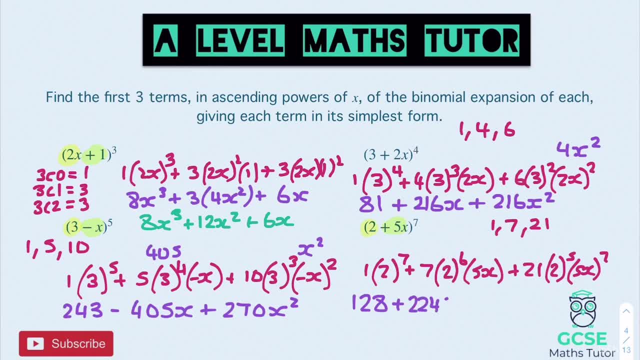 2240x for our first one and then for our last piece here. 2 to the power of 5 there in the bracket is 32, multiply that by the 21 is 672, and then obviously we've got 5x. 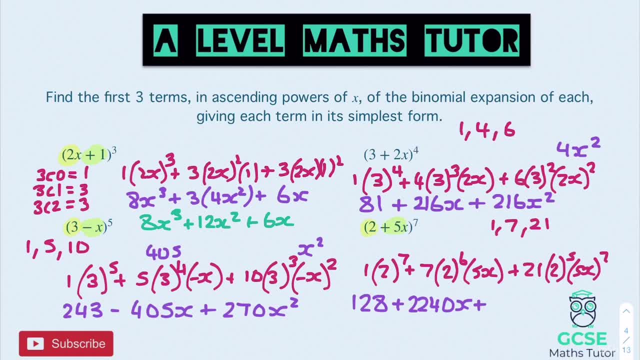 to the power of what's that last one there? 5x to the squared there. so 5x squared is 25x squared, so we've got 672,. we'll times that by the 25 now and we get 16,800,. 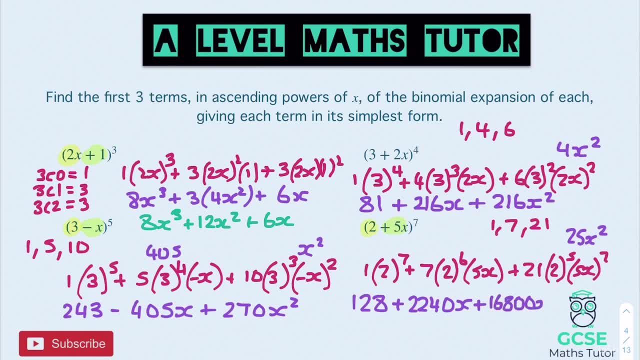 there we go. 16,800 x squared. there we go. so obviously some quite big numbers in this one. so don't let the big numbers put you off. sometimes you'll have to get very large numbers, but obviously you've got your calculator. 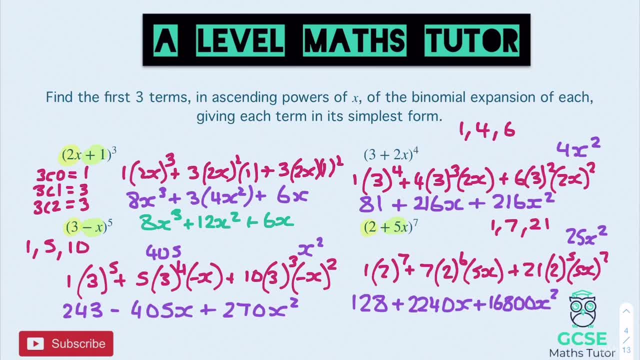 so all you've got to do is type in 21 times 2 to the power of 5, times the 25 there, obviously just making sure you are careful with the brackets in those scenarios there. obviously there was a couple of times that. 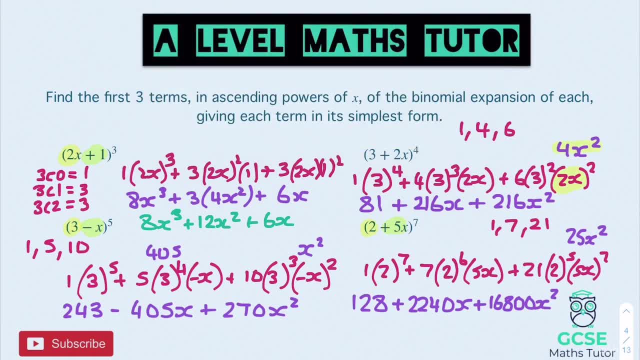 came up here we had the 2x that was being squared, that made the 4x squared, and the 5x here that was being squared, that made the 25x squared. obviously, just being careful with what coefficient of x that you are actually multiplying by there. 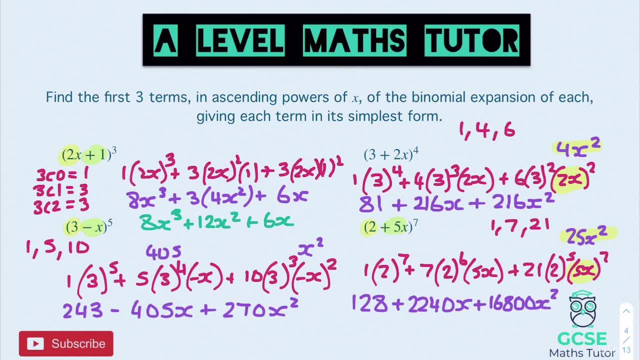 But there we go. that is obviously some of the binomial expansion there, where we've just got not necessarily nasty pieces in the brackets. but we're going to have a look at some now where we have fractions in the brackets and how we go about. 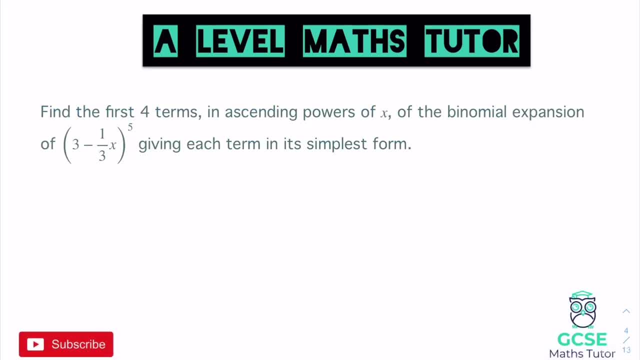 dealing with those as well. so let's have a look at that. Okay, so this question says: find the first four terms, in ascending power of x, of the binomial expansion of 3 minus a third x to the power of 5, giving each term its simplest form. 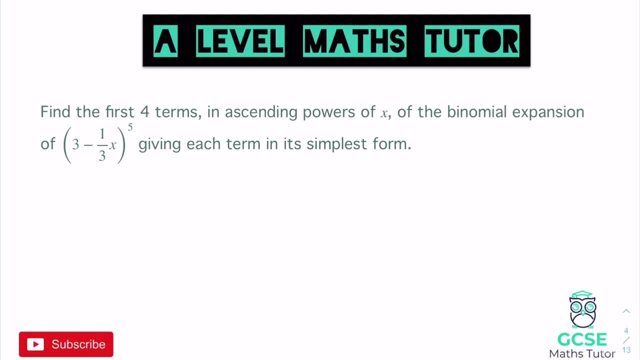 So let's have a look at this one. now we've got a power of 5, so before we start dealing with the fractions and having a look at how we're going to deal with that, we'll find the first four terms in the pattern here. 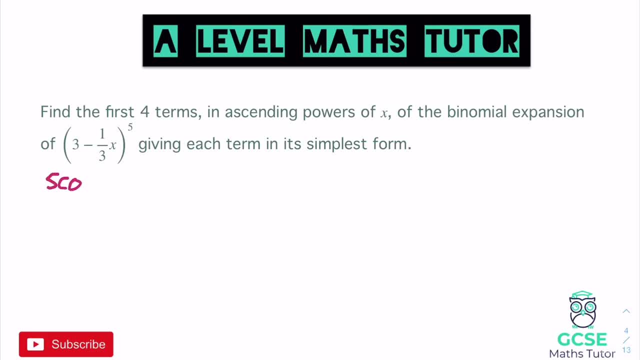 So we'll go for 5c0, 5c1, 5c2 and 5c3 and just work out what that pattern actually is now, obviously, we know the first one's 1, so we go for 5c1. 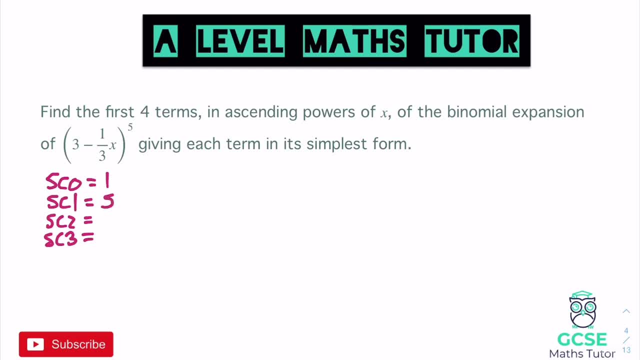 which is 5, the next one, 5c2, is 10, and the next one, 5c3, is also 10, there we go. So that's how many lots of this pattern we're going to have now. this time the first piece in our pattern is a 3. 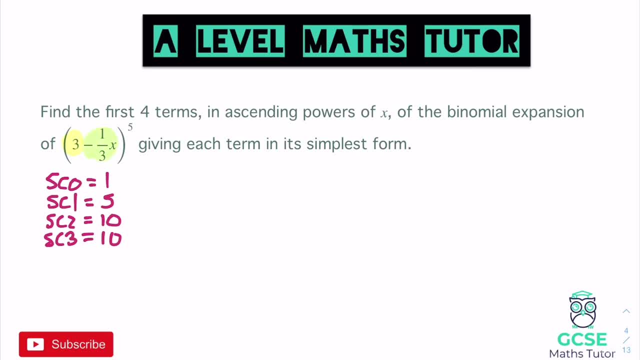 that's okay, and the second piece in our pattern is negative. a third x now. obviously that's okay as well, but we're just going to have to be careful when we're typing this into the calculator. another way that you could write this here is you could write negative. 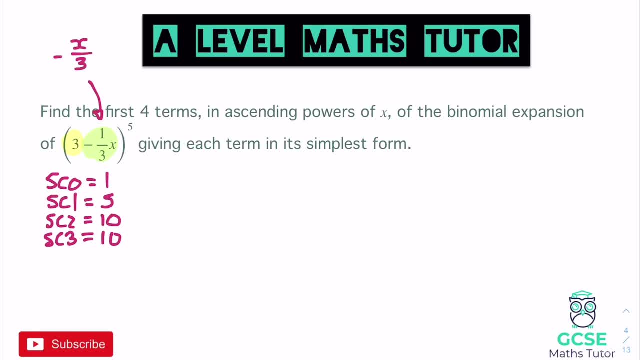 x over 3, so you could relieve it as that as well. I might actually write it as negative x over 3 instead, just to sort of make the terms a little bit easier to write. But let's go for this then. so we have one lot of. 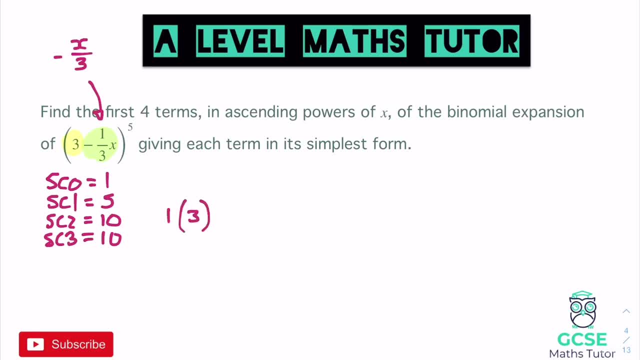 the first piece, which is 3 to the power of 5. so we've only got 3 more to do now and we're going to add to that. we've got 5 lots off for the next piece. let's just highlight these. 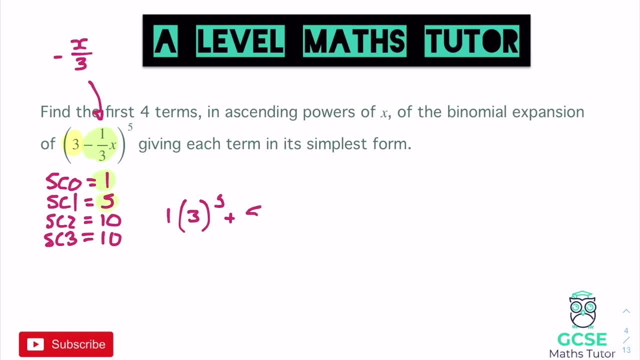 as we go. so now we're on this 5 lots, so we've got 5 lots off and we have 3 to the power of 4, and then we've got this negative x over 3 as well, so negative x over 3. 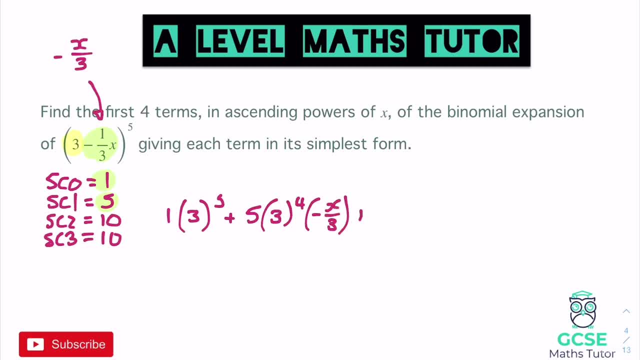 there we go on to the next piece again. so we have 10 lots of this one, so we've got 10 lots off. so we've got 10 lots off and we've got 3 getting down to the power of 3, and then we've got this negative. 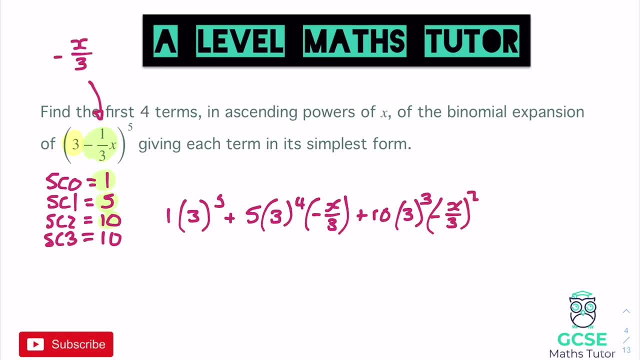 x over 3, which is now being squared. there we go, and then for our last piece, here again, we've got 10, lots of this. so we have 10, lots of 3, going down to the power of 2, and we've got. 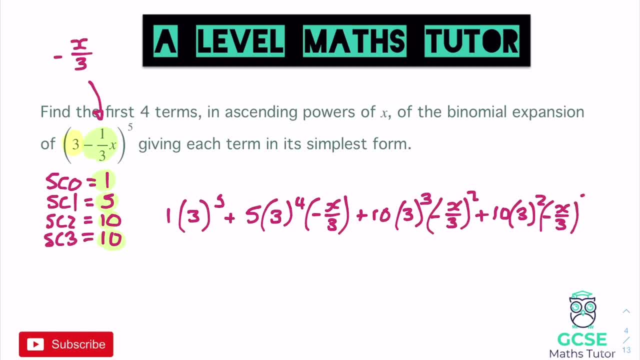 the negative x over 3, which is now going to be cubed right. so let's deal with all these pieces and the first one's ok. we've got 3 to the power of 5, we can work that out nice and easy. 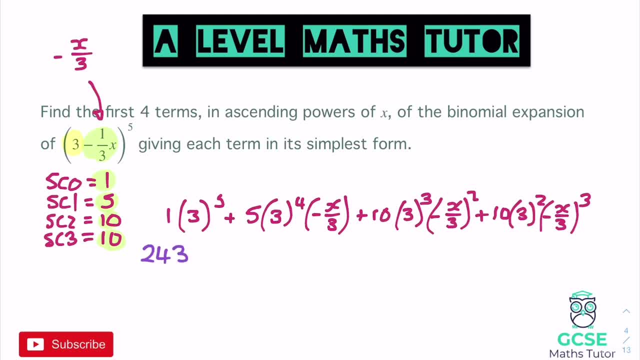 that's 243. so 243 is our first one, and we tick these off as you go. so that's done. the next one: 5 times 3 to the power of 4. let's work that out to start with. that's 405. 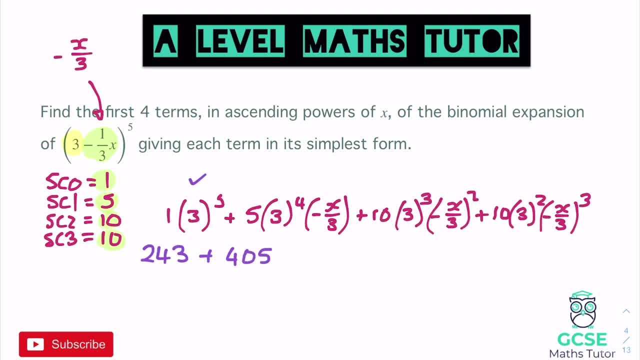 so 405, and that's going to be multiplied by negative x over 3. we'll come back to that and deal with that in a sec. on to the next one. so we have 10, lots of so, 10 lots of 3 cubed. 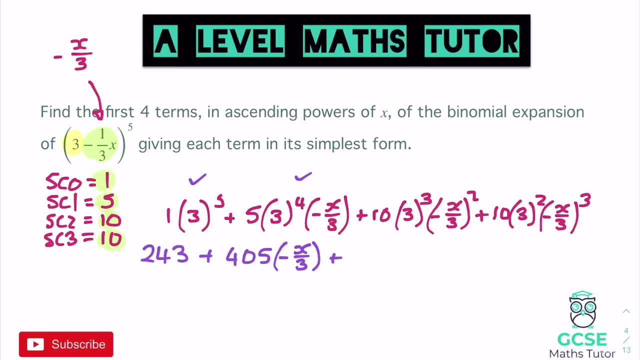 so we have 3 cubed, which is obviously 27 times that by 10 is 270. so we have plus 270, lots of- let's have a look- negative x over 3,. well, if we square that's going to become positive. so we're going to get x squared. 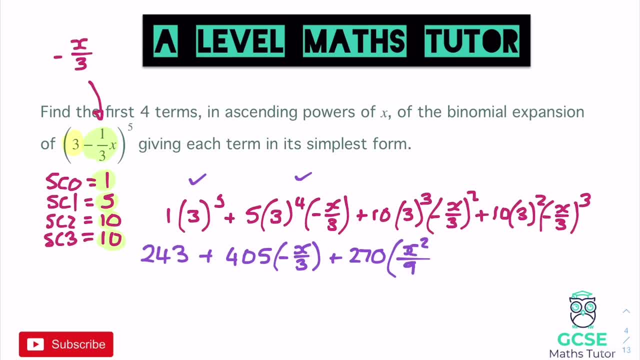 on the top and on the bottom, 3 squared is 9, so x squared over 9. there we go, and that's that pieced out with and on to the next one, obviously just being careful with those when you're squaring that. 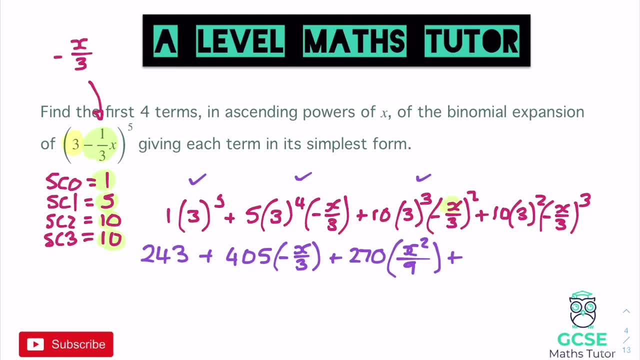 remembering that's going to make it positive. so we get the x squared on the top, positive x squared 9 on the bottom, on to the next one. 10 times 3 squared is 90. so we've got 90 and that's going to be, and we've got negative x. 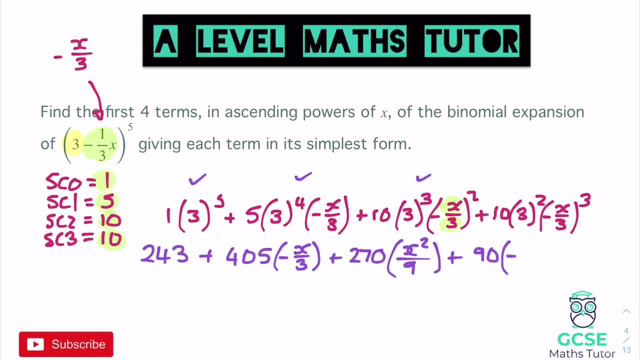 over 3 cubed. so when we're cubed it's going to stay negative. so we're going to have negative x cubed on the top and 3 cubed, which is 27, on the bottom. there we go and that's the. 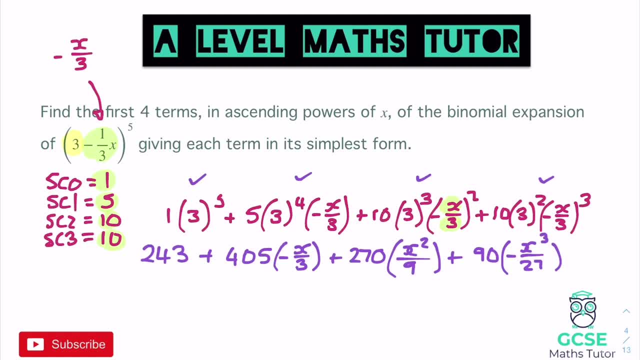 last pieced out with right now, simplifying all of this then. so we've got 243 at the start. that's all good, and then we've just got to be careful on this next bit now. negative x over 3. obviously we could have had the negative a third there. 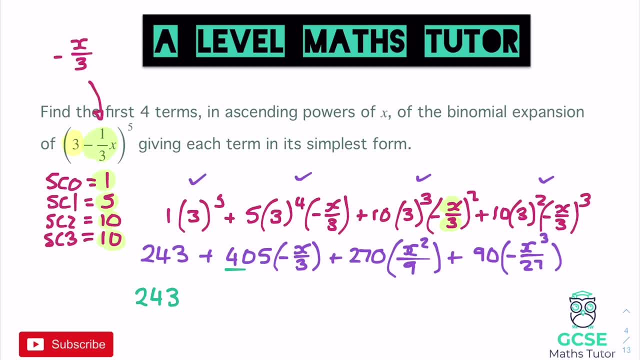 we basically just want to do a third of 405, so if we do a third of 405, we have 405 divided by 3 is 135 and obviously it's negative there. so it's going to be negative 135 x. there we go. 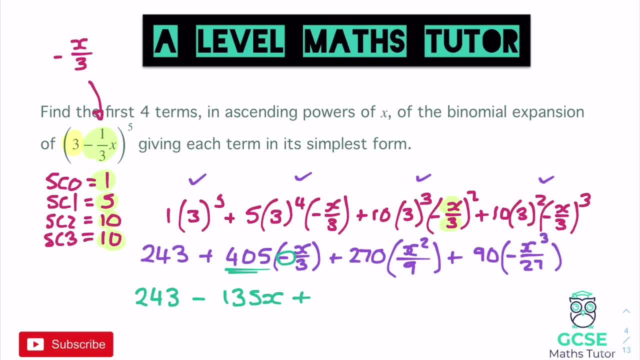 on to the next piece. we have 9 on the bottom there, so we want to divide that 270 by 9. obviously it's positive this time, so we'll divide that by 9. 270 divided by 9 is 30, so we get 30x. 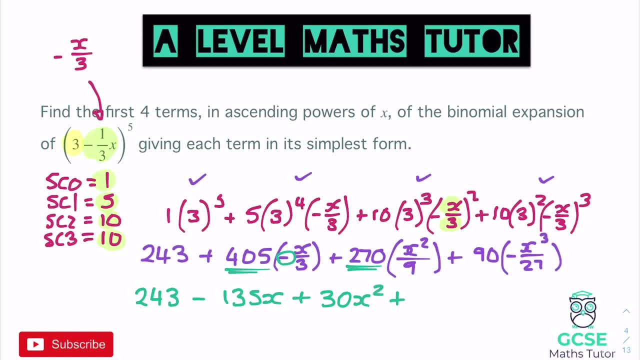 squared on to the next piece. 90 divided by 27 is not as nice. it gives us a fraction here and we've got to be careful because it's negative. so that's not going to be plus there, it's going to be minus. 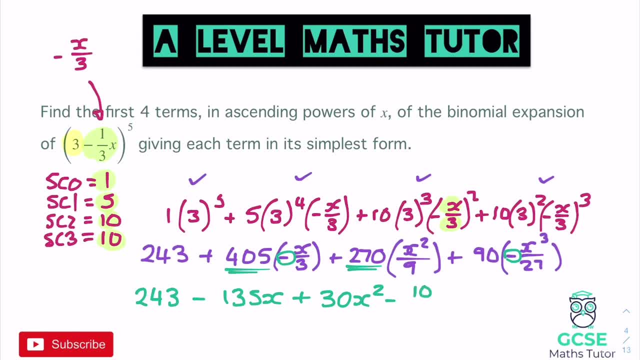 so we get minus 10 over 3, which is what 90 divided by 27 comes out, as with an x cubed. there we go, and that is those first four terms finished. so obviously just be careful on this, because obviously sometimes you can get these fractional. 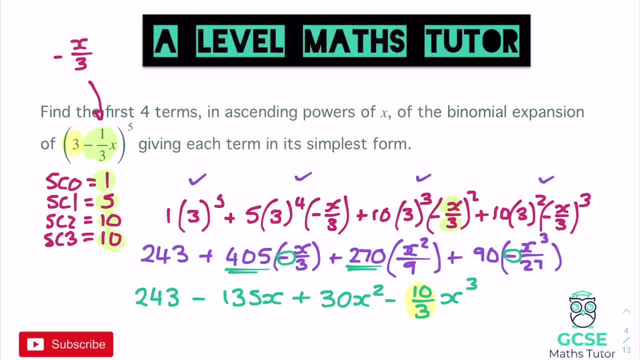 pieces or these fractional coefficients here, and that is quite common on these questions. so you just need to be nice and careful, obviously just watching out for any pieces here that are negative like the two there, just making sure that you show those with your negatives here as well. 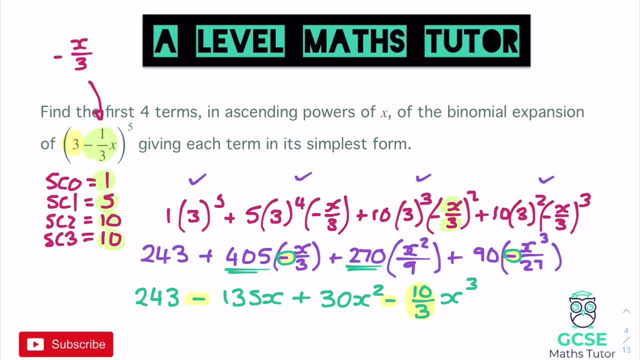 when you do have these fractions involved. just remember, obviously you're just finding a fraction of that coefficient. there again, it's just like 405 multiplied by negative, a third in terms of actually getting these coefficients. so here we've got the 135, a third of that. 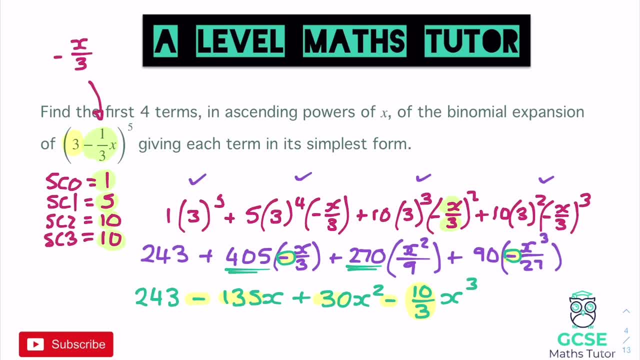 and one ninth of 270 gives us the 30. obviously our fractional piece at the end as well there. so just being careful, there's the first four terms and ascending powers of x, and we've simplified each term, so obviously don't be put off by these fractions within the brackets. 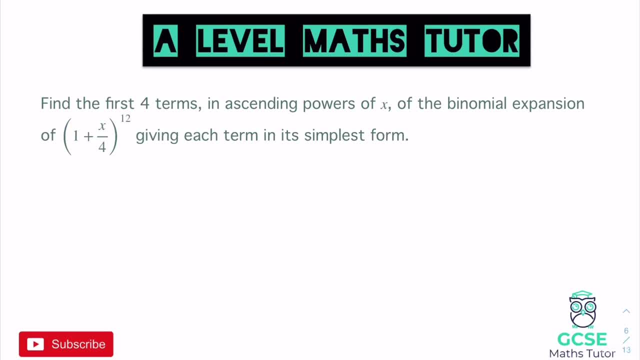 we're going to have a look at one more of these before you have a go. so this one here is very similar. it says: find the first four terms and the ascending powers of x of the binomial expansion of 1 over 1 plus x over 4 to the power of x over 4. 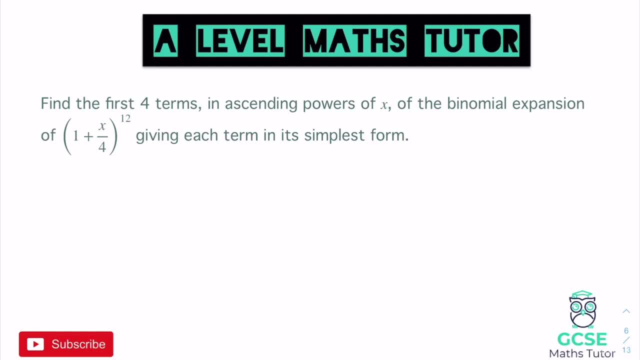 1 plus x over 4 to the power of 12 and again giving it in its simplest form. so we've got a power of 12 this time, which doesn't look very nice. but if we start putting them in, 12c0 is obviously 1. 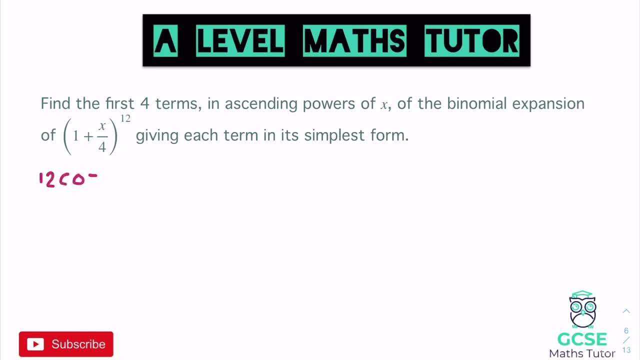 so just power of 12. so our first one in that list there is 1. we have 12c1, which is 12. we get 12c2 again. let's just type this into the calculator: 12c2 is 66, so it's looking quite nasty now. 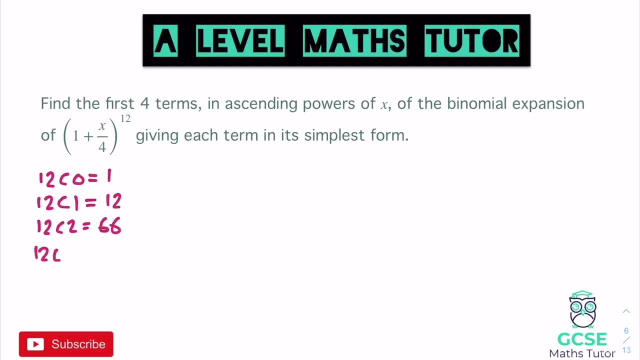 and 12c3, which is 12c2, which is 220. there we go. definitely doesn't look very nice on this particular question here, so obviously, going ahead with this then and finding all these terms, let's see what we get. so we have 1 lot of 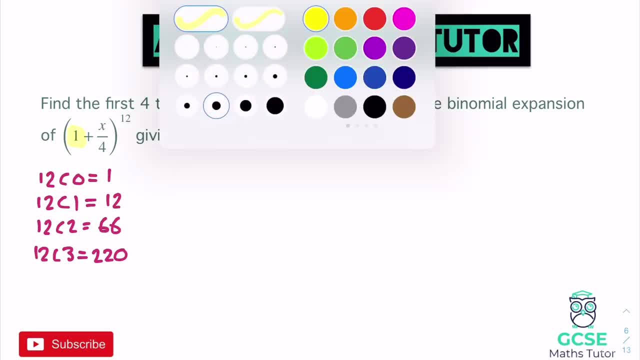 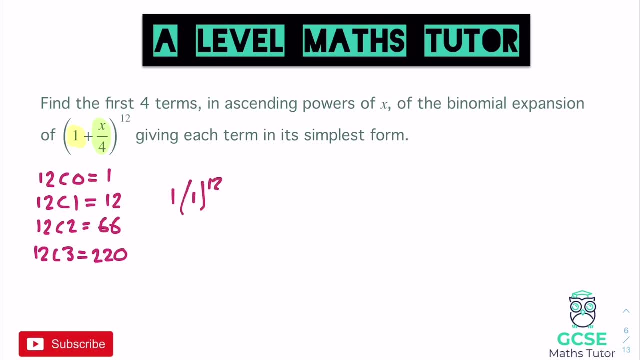 and again our pieces are 1 and we have positive x over 4, so we've got 1 lot of the 1 to the power of 12. we're going to add to that, just moving down our list here. now we're on the 12 lots. 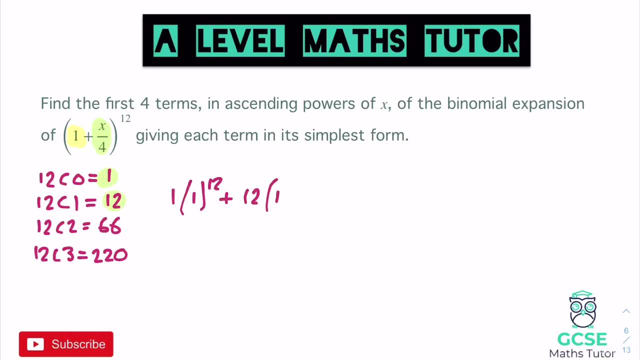 so now we have 12 lots of 1 to the power of 11, and we have the x over 4. there we go on to the next piece. we have 66, lots of this one. so 66 lots of 1 to the power of 10. 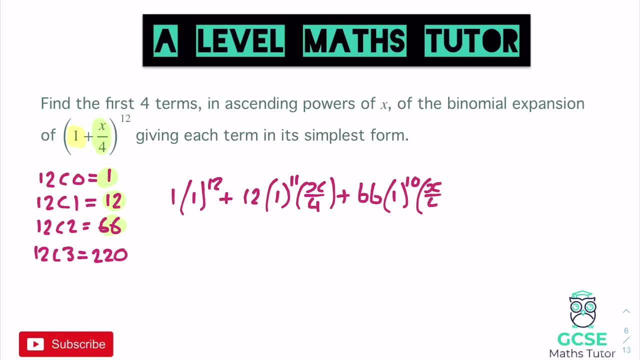 and then x over 4 squared, and then for our last piece here, which we have 220, lots of. so we have 220 lots of 1 to the power of 9 now, and x over 4 to the power of 3. right, there we go. 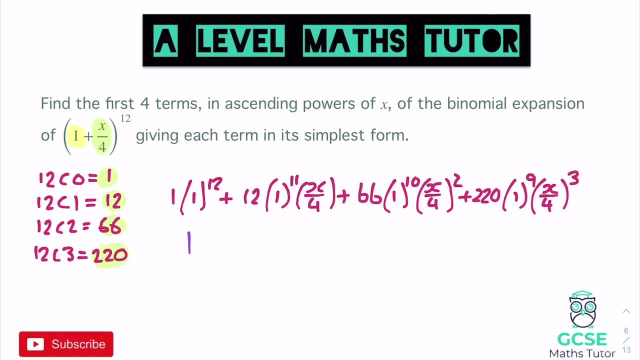 and let's just go about simplifying all of this. so 1 to the power of 12 is 1. this is quite nice, because we get these 1s here. so 12 times 1 to the power of anything, that's just going to stay as 12. 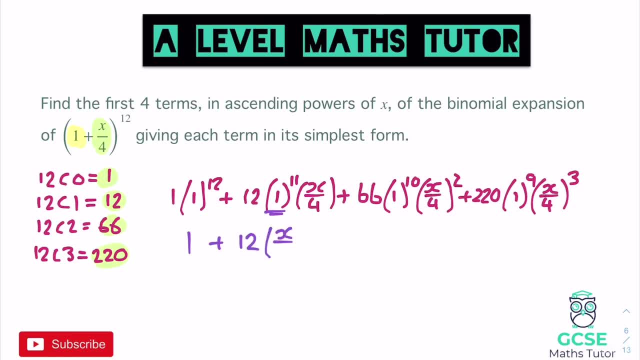 so we have 12 lots of x over 4, then we have 66 lots of, and we've got x over 4 squared, which is x squared over 4 squared, which is 16, and then, for the last one, 220 times 1 to the power of 4. 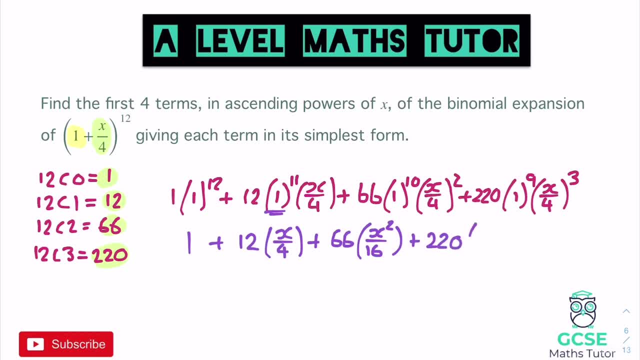 x over 4 squared, x over 4 squared, x over 4 squared, which is 1 to the power of 9, is 220. so 220, lots of, and we get x cubed over 4 cubed and 4 cubed is 64. 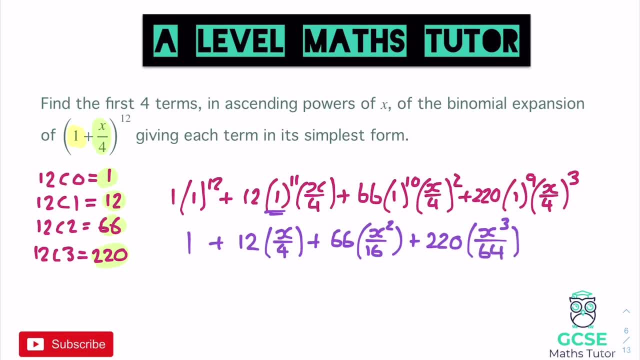 so it's x cubed over 64. there we go, and then, obviously, just simplifying this down again, 1 at the start stays as 1, 12 divided by 4. there, obviously, we're doing a quarter of this, so that's 3, so 3x. 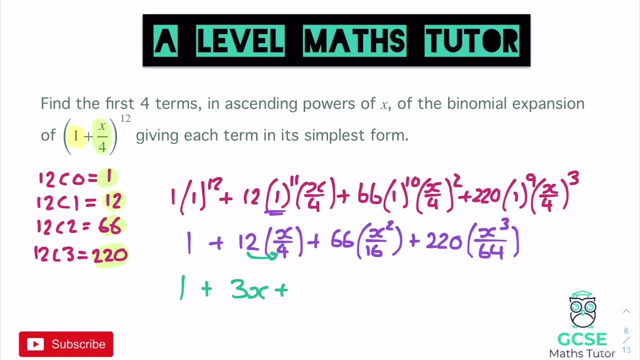 then we have 66 divided by 16 for this next piece, which is 33 over 8. not very nice. so we've got 6 divided by 16, so we get 33 over 8- lots of x squared. and then we've got the last piece there. 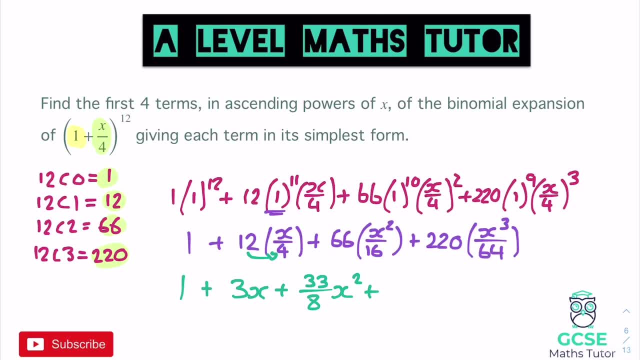 which is 220 divided by 64, which gives us 55 over 16 as a fraction. so 55 over 16, x cubed. there we go. so, as I said, again we're getting these fractional coefficients of x squared and x cubed there. but again, that shouldn't put you off. 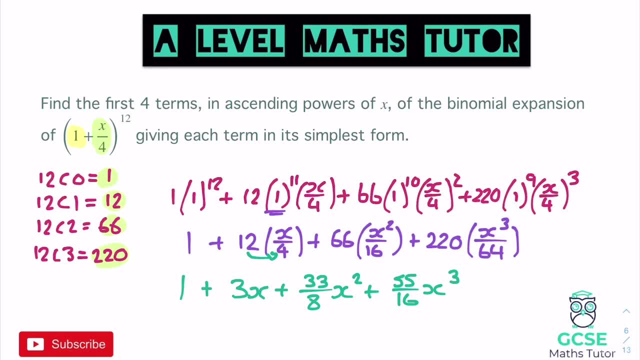 obviously we're just typing it into a calculator. so 66 over 16 just gave us that 33 over 8 and that's 55 over 16. okay, but there we go. there's our final answer. there is the first four terms and ascending powers of x. 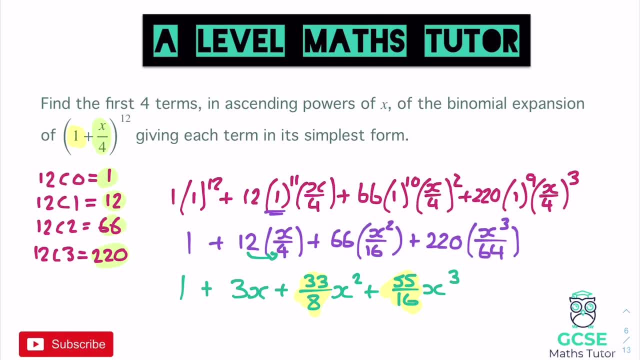 and obviously just showing you there not to be put off by these fractional pieces. but there we go. we're going to have a couple of questions for you to have a go at, so let's have a look at those now. okay, so here's your two questions. 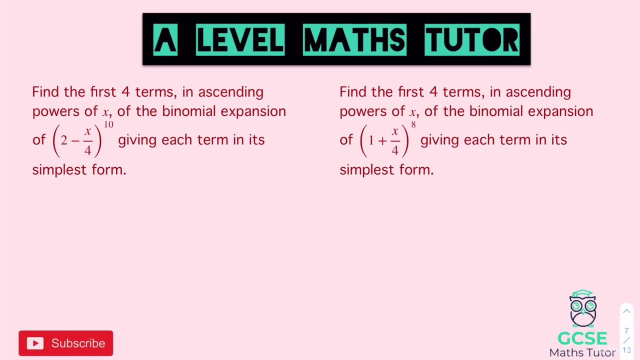 so pause the video there. have a go. we'll go over the answers in a sec. okay, so for this first one, then our first piece is 2 and our second piece- there is negative x over 4, so obviously we've got a power of 10 there. 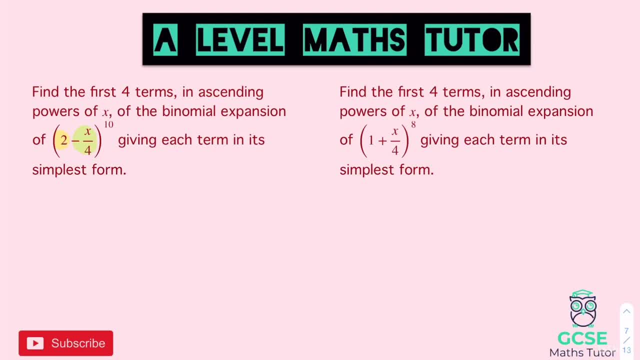 and we're finding the first four terms. so we'll do 10c0, which is 1, 10c1, which is 10, 10c2, which is 45, and 10c3, which is 120. there we go. so there's our first four terms for the pattern. then. 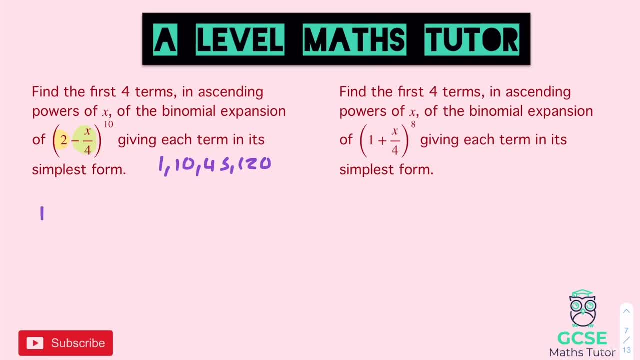 or first four pieces of the pattern. so we have one lot of the 2 to the power of 10. we're going to add to that. we've got 10 lots of 2 to the power of 9, and then we have the negative x over 4. 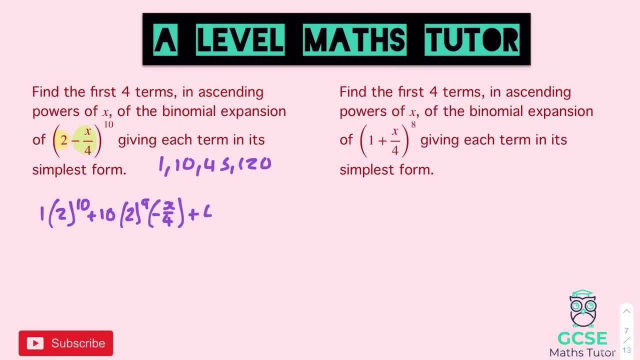 then for our next one, we've got 45 lots of this one, so 45 lots of 2 to the power of 8, and then we have the negative x over 4, which is all going to be squared. and then for our last piece there, 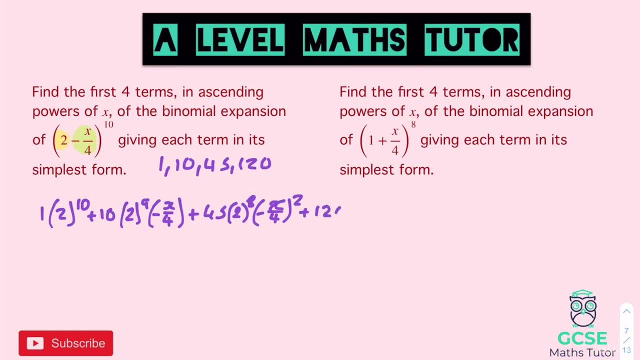 we're going to have 120, lots of. we have 120, lots of. let's have a look: 2 to the power of 7, and then we have our negative x over 4, which is going to be up to the power of 3. right, there we go. 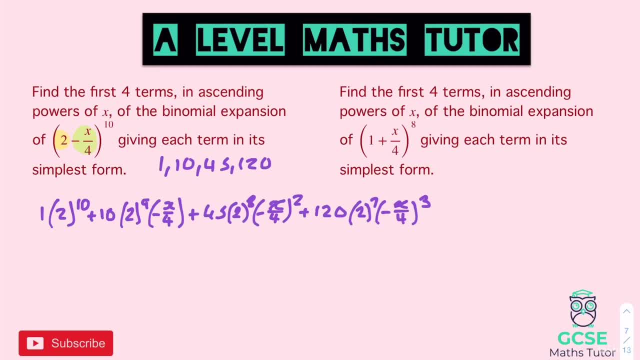 so that's our first four. we just need to simplify this down. so 2 to the power of 10. I'm just going to do that on the calculator. here's 1024, so 1024 plus 10. lots of 2 to the power of 9. 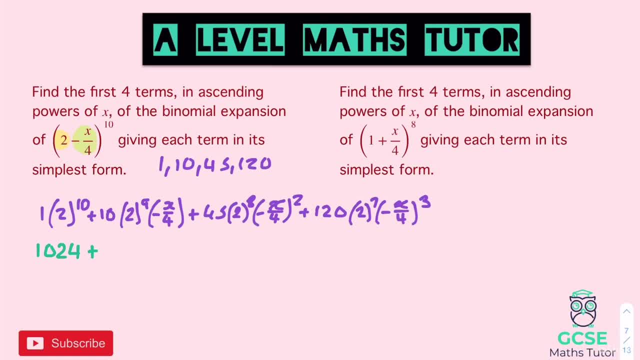 so 10 times 2 to the power of 9. let's have a look what that comes out, as. that comes out as 5120. so 5120 and that's obviously being multiplied by negative x over 4, then we have 45. lots of 2 to the power of 8. 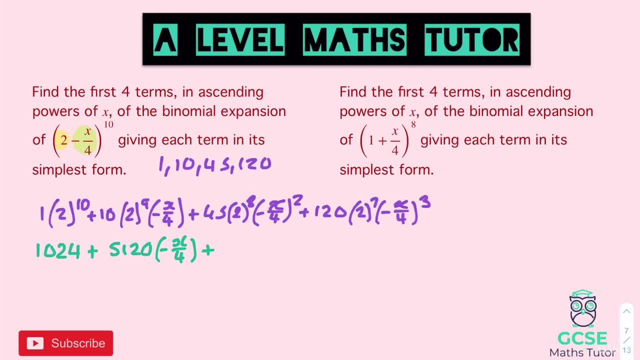 so 45 times 2 to the power of 8 is 11520. there we go, and then we have the negative x over 4, which is being squared. so negative x over 4 squared. so I think about what that is. that's going to be positive x squared over 16. 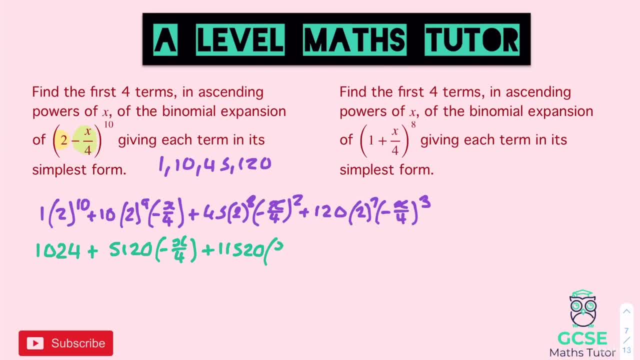 so we have positive, because it's negative- being squared. so we have x squared on the top and 4 times x over 4 squared is 1025 And 4 times 4 is 16 on the bottom. There we go 120 times 2 to the power of 7.. 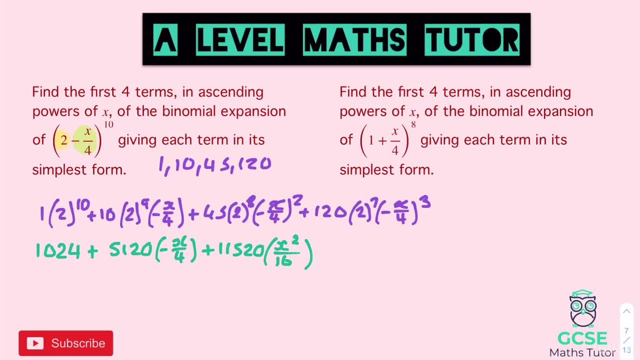 Let's work that out: 120 times 2 to the power of 7 is 15,360.. So plus 15,360.. And then we have in the bracket there, negative as it's being cubed, X cubed on the top. 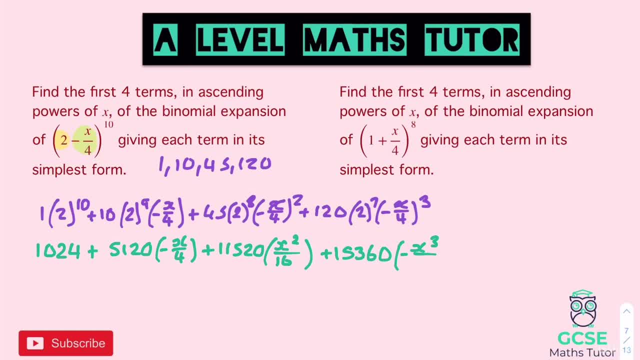 4 cubed on the bottom. 4 cubed is 64.. So 64 on the bottom. There we go, And then we just need to tidy all of this up. So let's have a look at what we get. We've got the 1,024 at the start. 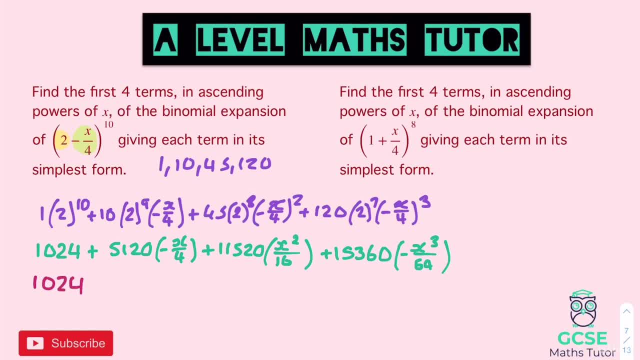 So 1,024.. Then we've got 5,120.. We've got x over 4.. So we need to divide that by 4.. So 5,120 divided by 4 is 1,280.. And that's going to be negative with the x there. 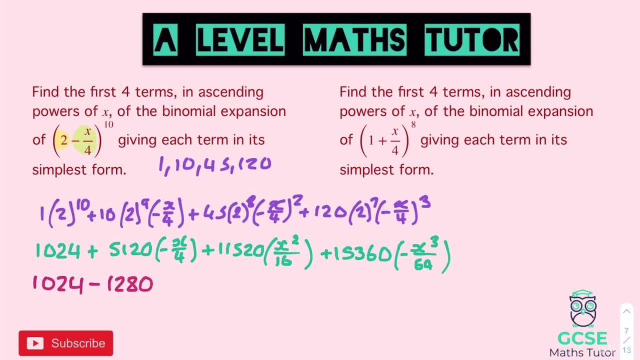 So negative 1,280x. Then we're going to add to that The next piece is going to be positive. So 11,520 divided by 16 is 720.. So plus 720. And we've got x squared. 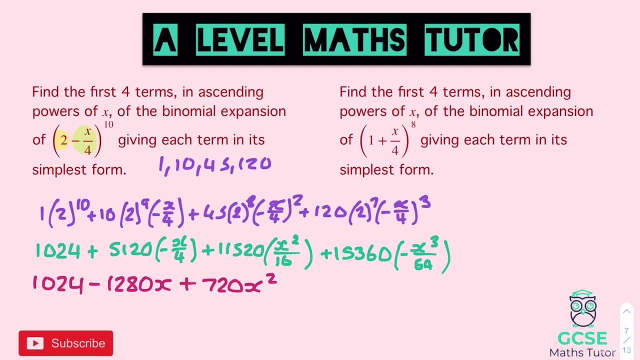 There we go And for the next piece, we've got 15,360.. We're dividing that by 64 this time, which is 240.. And it's a minus over there, So being careful with that, So we've got minus 240x cubed. 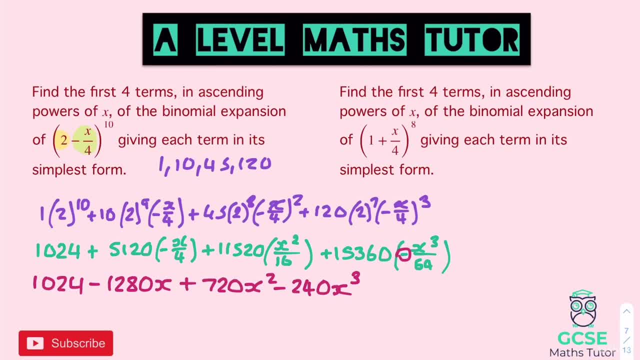 Right, there we go, And that is our first question there completed Right now. we're going to need a bit of space for the next one, So I'm going to get rid of all this working out. Let's get rid of that. 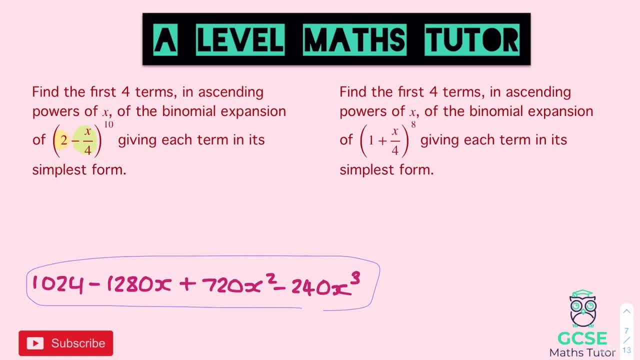 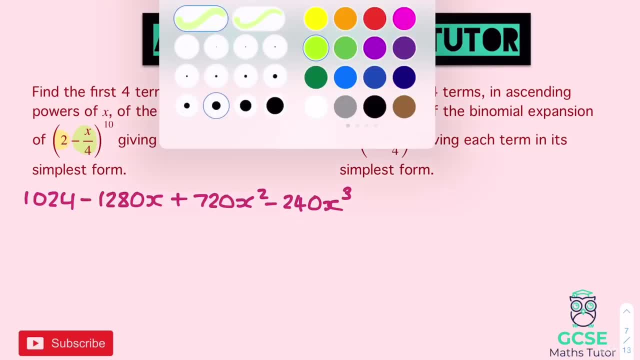 There we go, And we'll move this up. That one's finished. There we go. OK, so on to our next one. Now for our powers, for this one, then. let's have a look. Now for our first piece. there we have a 1.. 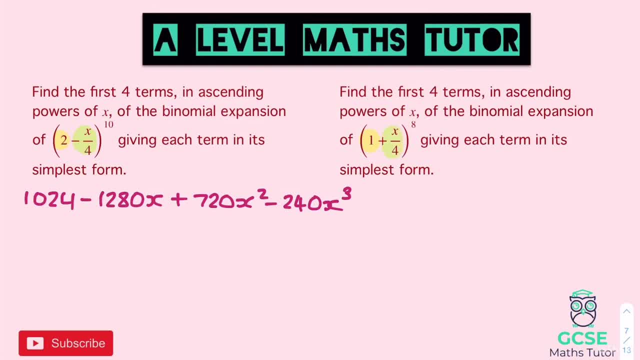 And for our second piece. there we've got positive x over 4. And it's a power of 8. So if we do 8c1,, 8c0, and 8c1.. Let's have a look. 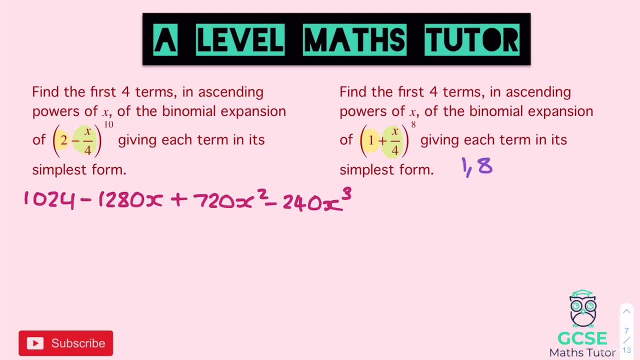 That's 1, then 8.. 8c2 is 28.. And then, for our last one there, 8c3 is 56.. OK, so we've got 1 lot of. I'm going to do this down here. 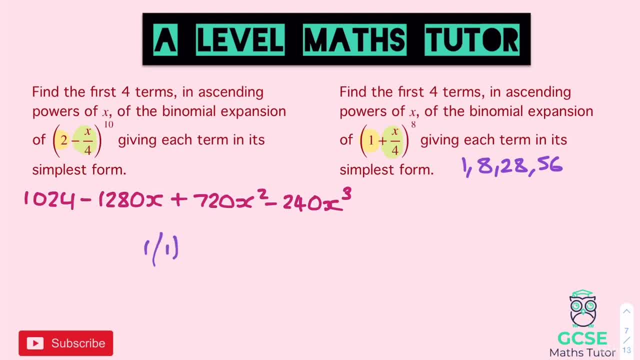 So we have 1 lot of the 1 to the power of 8. Then we have 8 lots of the 1 to the power of 7. And then the x over 4. And then we have 28 lots of. 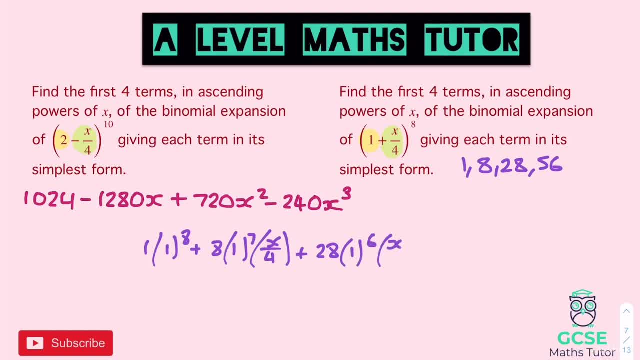 1 to the power of 6.. And then the x over 4 squared, And then for our final piece here, which we have 56, lots of. We've got 56 lots of 1 to the power of 5.. 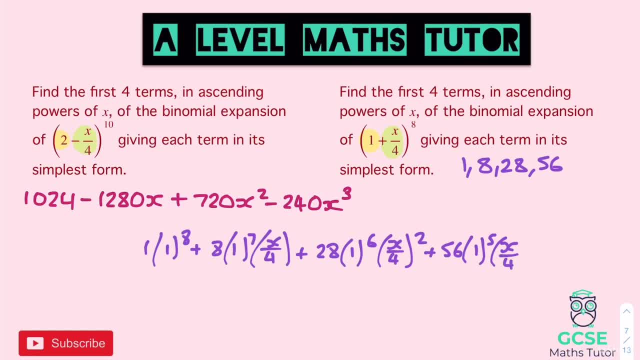 And the x over 4 to the power of 3.. OK, so let's simplify this down. Let's see what we get: 1 to the power of 8 is 1.. And we've got 8, lots of 1.. 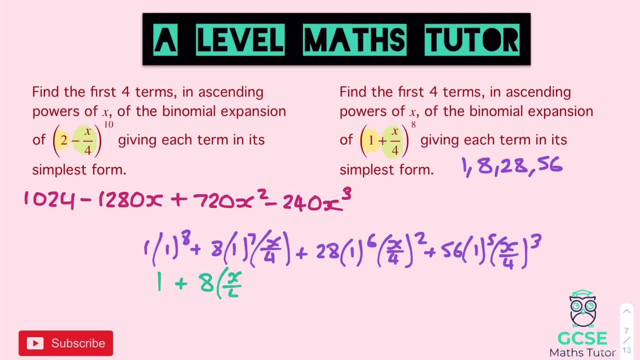 So that's 8 lots of x over 4.. Then we have 28 times 1, which is 28 lots of, And we've got x squared over 16 on the bottom. There we go, Squaring x over 4.. 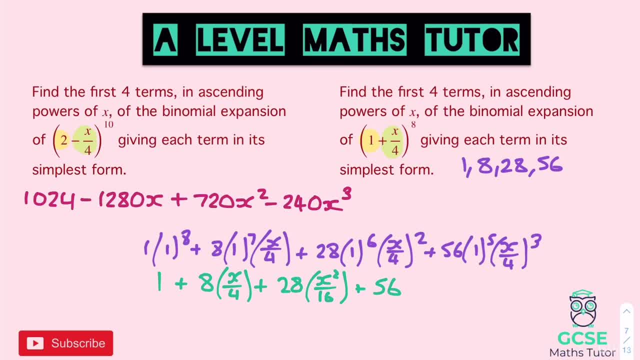 And then we have 56 times 1, which is 56. So 56, lots of. And then we've got x cubed on the top over 64. And there we go. Right, that was quite nice and easy actually to just expand those pieces because of that 1 in there. 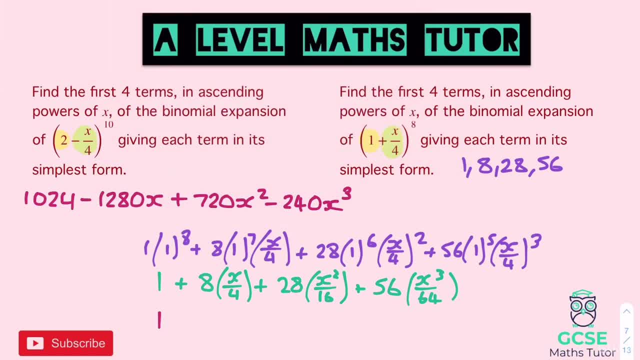 Always makes it quite nice. So to finish this off, then we've got 1 plus 8 divided by 4. There which is 2. So 2x 28 divided by 16. Let's do that on a calculator. 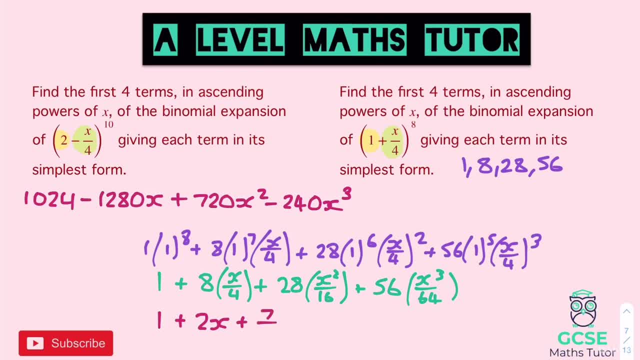 That gives us 7 over 4.. So we get plus 7 over 4 x squared. And for our last one there we've got 56 divided by 64, which gives us 7 over 8. So plus 7 over 8.. 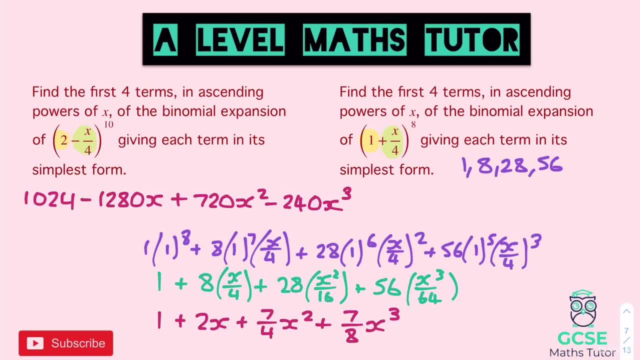 And then that's with the x cubed there, There we go, And there's our final answer. OK, so there we go. We had 1,024.. Take away 1,024.. 280x plus 720x squared minus 240x cubed for the first one. 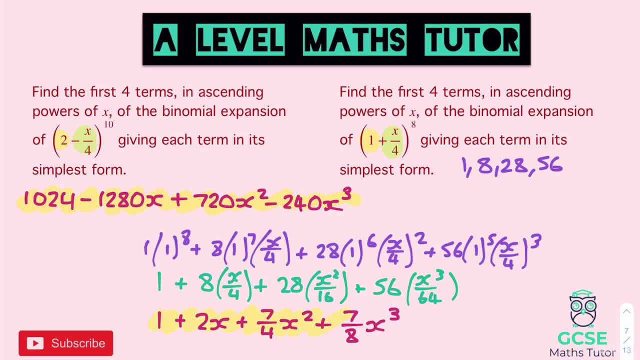 And then for our final one, here we had 1 plus 2x plus, And then we've got some fractional coefficients: 7 over 4x squared and 7 over 8x cubed. And there we go. There's our final answer. 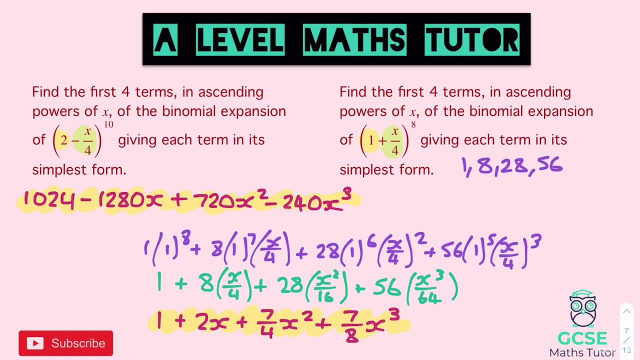 Obviously, just being careful with those fractional pieces and just being careful, Obviously all we need to do is type these into the calculator as we go, So it shouldn't really throw you those sort of fractional pieces there, Because obviously your calculator will simplify that for you. 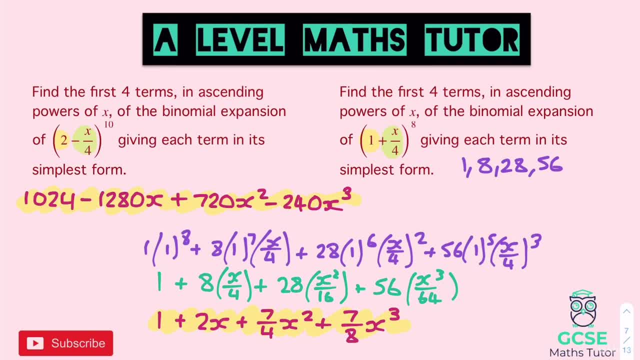 But there we go. So that is obviously some of this binomial expansion With And non-fractional pieces in the bracket and with fractional pieces in the bracket. Now we're going to have a look at some of these problems that we had a look at right at the start of the video. 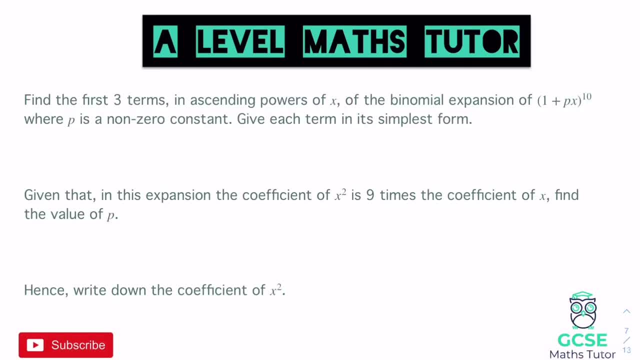 And have a look at how to solve those using these processes. OK, so this question says: find the first three terms in descending power of x, of the binomial expansion of 1 plus px to the power of 10.. It says where p is a non-zero constant and give each term in its simplest form. 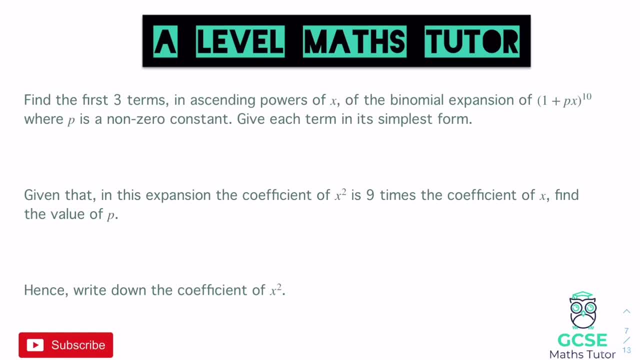 So, obviously, p is an actual number that we're going to find. Obviously, it hasn't asked us to find that yet. It's just asking us to find those first three terms. In the next part of the process, though, Or the next part of the question, it says: given that in the expansion, the coefficient of x squared is 9 times the coefficient of x, find the value of p. 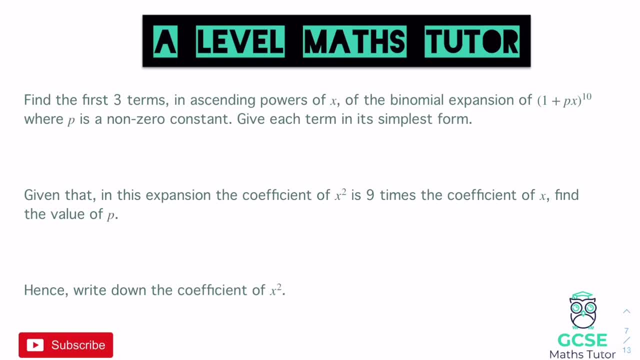 So we're going to find that value of p later on in the question And then it says: hence write down the coefficient of x squared. And we're just going to follow this step by step and have a look at how to approach this. 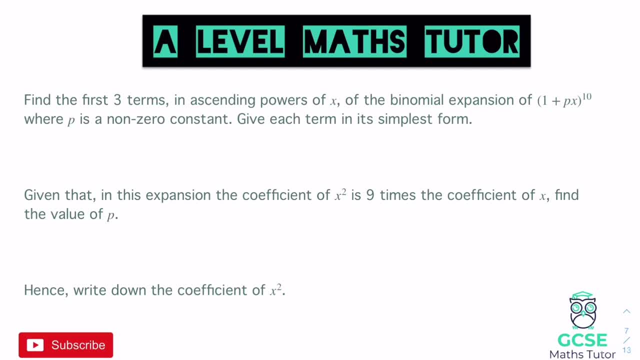 And then you've got one to have a go at. So, finding the first three terms, then We've got a power of 10.. And just bearing in mind, our first piece is a 1,, which is always nice, And our second piece is this: plus px. 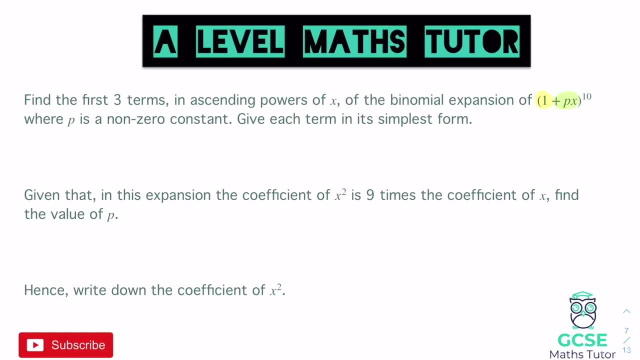 So, as we've got a power of 10, we need to do 10.. So we've got 10c0 to start with. So we've got 10c0, which is 1.. We're only finding the first three terms. 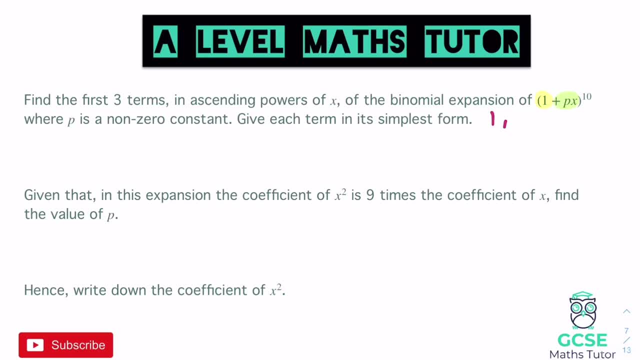 So we've got 1.. 10c1 is 10., And then we have 10c2, which is 45. There we go. So that's how many lots of each we're going to have on this particular one here. 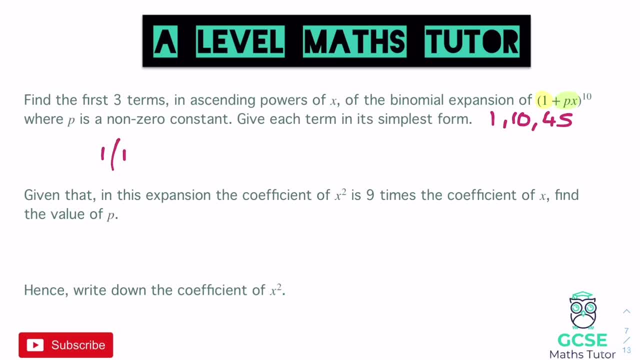 So for this one, then we've got one lot of, And then that's 1 to the power of 10, the first piece We're going to add to that. We've got 10 lots of, And it's 1.. 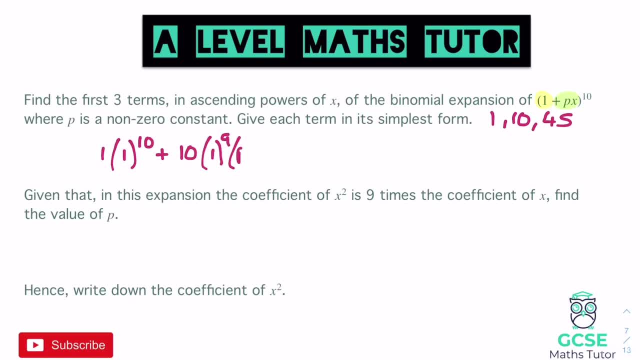 We're now 1 to the power of 9.. And then px as our second piece, And then, for the final one, we have 45 lots of 1 to the power of 8.. And then px to the power of 2.. 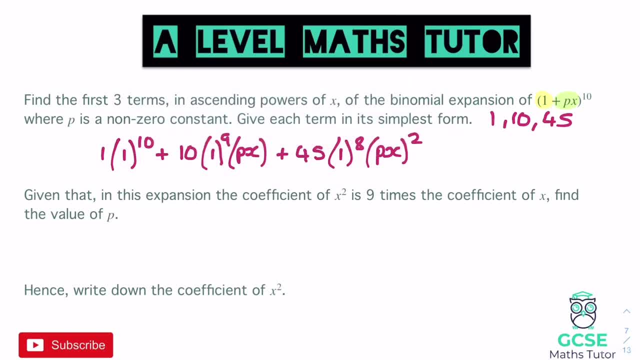 There we go Right. so if we simplify this down, then 1 to the power of 10 gives us 1 for our first piece. 10 times 1 and then times the px gives us 10px. So we have 10px for the second piece. 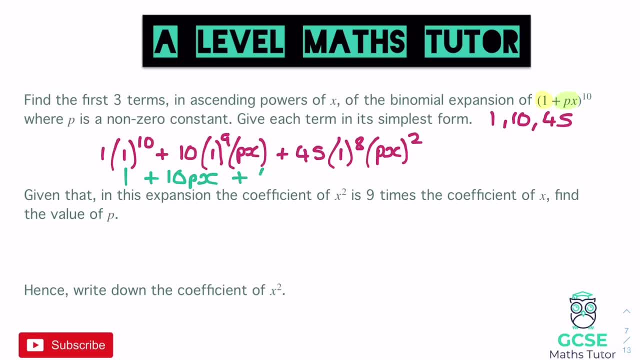 And then for our final piece: there 45 times 1.. 1 is 45.. And px, in brackets squared, squares both of those letters. So we get p squared, x squared. There we go Square in both of those letters. 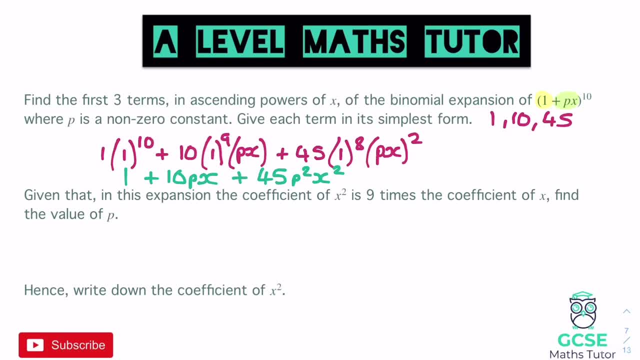 So 1 plus 10px, plus 45p, squared, x squared, And there's our first three terms in ascending powers of x. Now it says: given that in this expansion the coefficient of x squared is 9 times the coefficient of x, 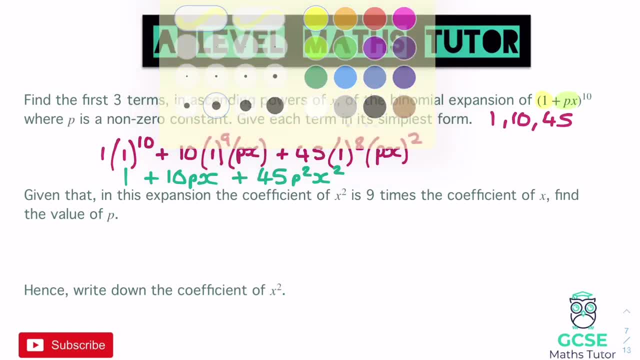 Well, the coefficient of x squared- let's have a look and let's highlight that- is 45p squared. That's what's in front of the x squared, And the coefficient of x is 10p. So what it's saying is OK if 1 is 9 times the other. 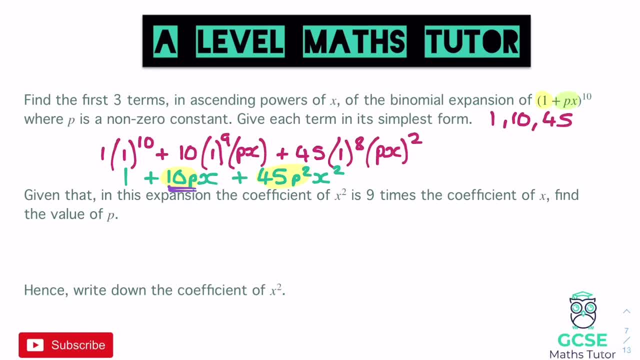 it's saying, if we multiply this coefficient here by 9, it would be equal to this coefficient here, Or in other words, 9 times 10p is going to be equal to 45p squared. Or you could do it the other way around. 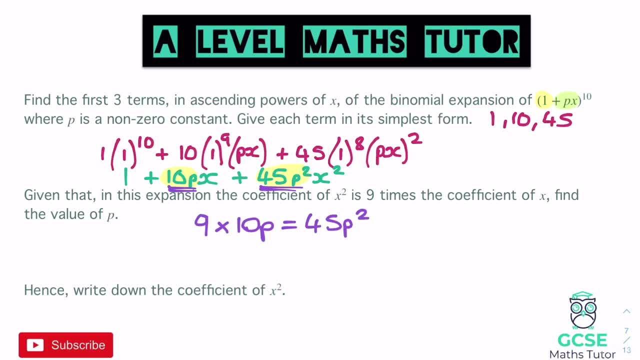 We could do. 10p is equal to 45p squared divided by 9.. Completely up to you which one you do. Obviously, 45 nicely divides by 9, so that would be quite a nice way to do it, But I'm just going to follow this process. 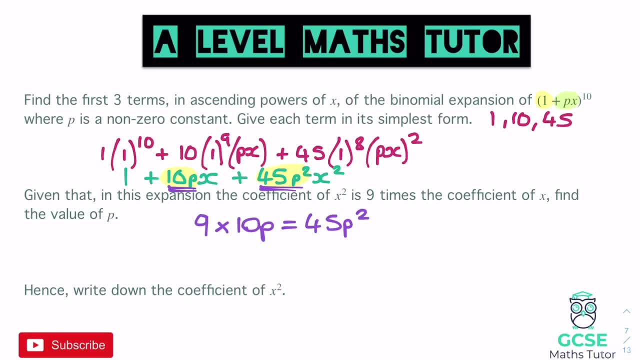 as I've written it down this way. now It doesn't really matter which way. It's probably easier actually to divide it by 9, because I think we're going to divide it by 9 anyway in a sec. But let's have a look. 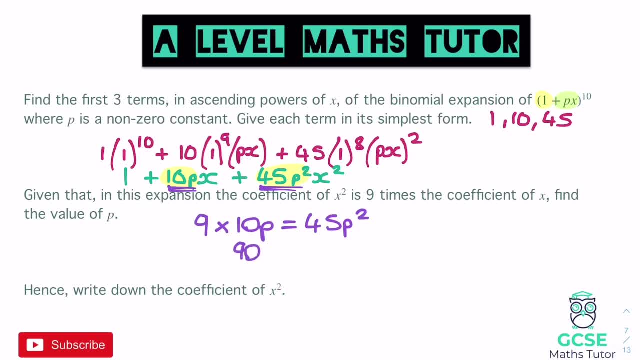 So if we times that by 9, anyway, we get 90p equals 45p squared, And then we just need to solve that as an equation. So dividing both sides by p would obviously remove the p from the one side, So we'd get 90 equals 45p. 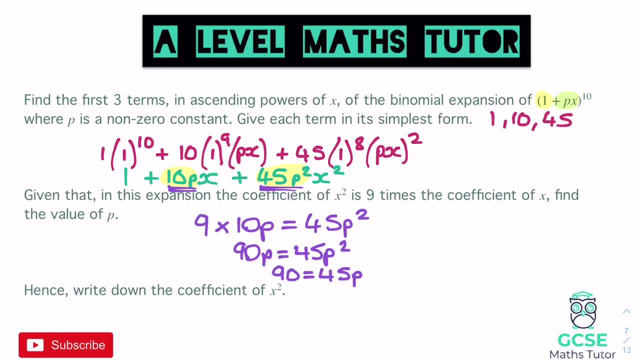 Just dividing both sides by p there. Then we could divide both sides by 9.. Or we could actually divide both sides by 15. Completely up to you. Or we could just divide both sides by 45, and that would tell us what p is. 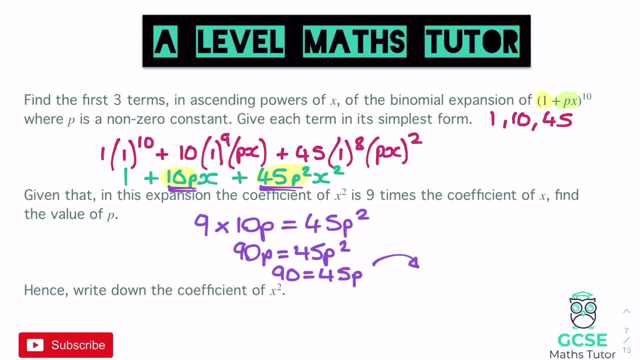 So if I divide both sides by 45, just write that down: Divide by 45. As we've got 45p there, we get 2 equals p or p equals 2. And there we go. There's our answer for that part. 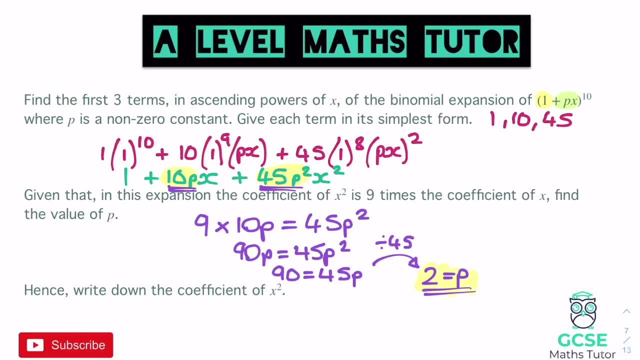 So p equals 2 or 2 equals p. Then it says: hence write down the coefficient of x squared. Well, the coefficient of x squared is 45p. There we go, And we now know that p is 2.. So that's 45 multiplied by 2 squared. 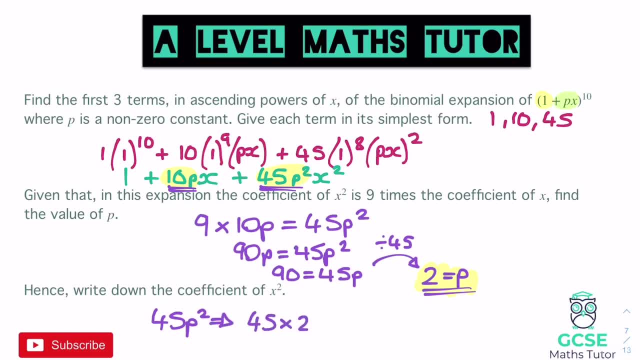 which is 45 times 4.. And 45 times 4 is 180.. And there we go. There's our coefficient of x squared 180.. Right, there we go. So there's our final answer. So, in terms of actually what we did there, 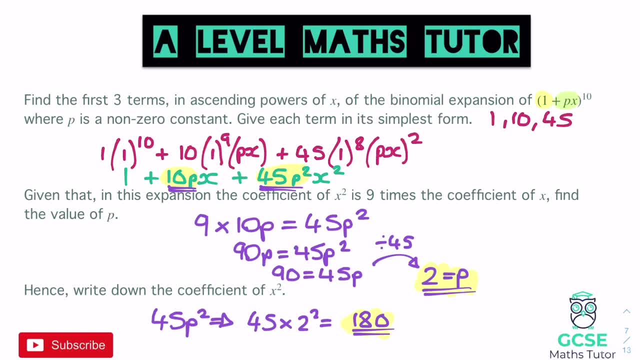 obviously we had a different piece within our bracket. We had a px. I'm just being careful with that. I think the point in a way, you need to be careful with it is obviously this bit here where we get the px. So we've got the px. 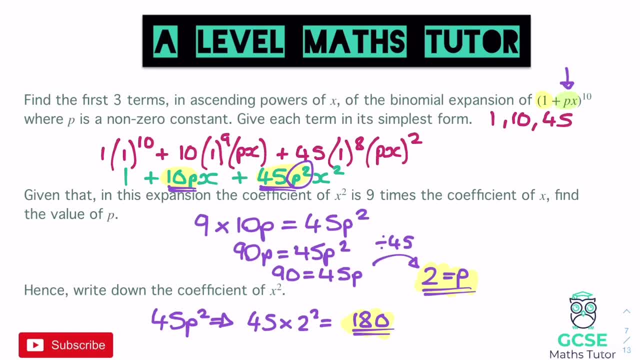 We've got the px. We've got the px. We've got the p squared, x squared, I think. other than that, the rest of it was quite nice and simple. And then, obviously, just reading the wording carefully, it said: one coefficient was 9 times the other. 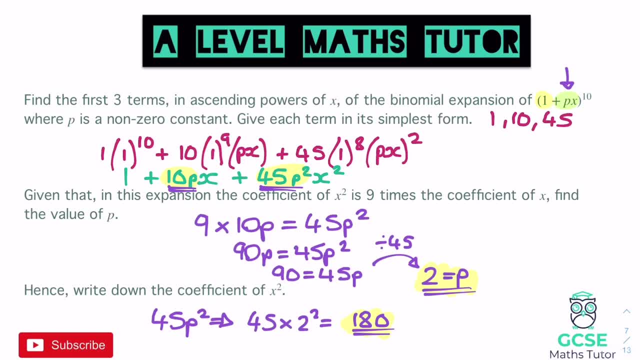 So obviously multiplying that by 9 or dividing the other one by 9 there gave us a little equation to solve. We got our value of p and then subbed that in to find the coefficient of x squared. So hopefully nothing too horrible there. 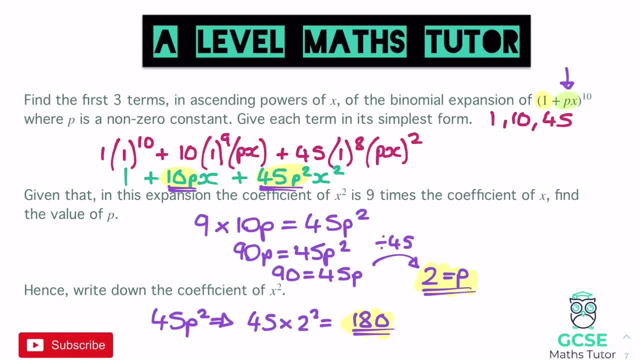 But obviously here's a question for you to have a go at, And then we've got one last one to finish on, So let's have a look at that one now. Okay, so here's your question, So have a read of this one. pause the video there. 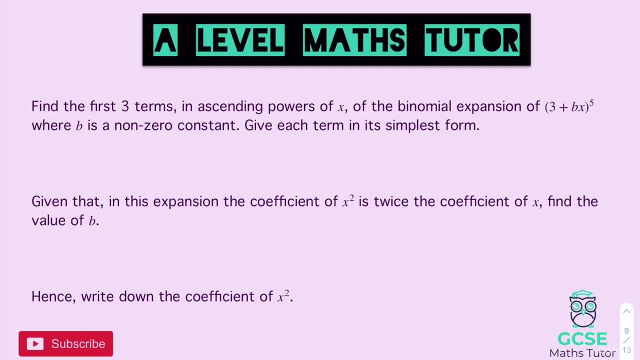 Okay, so finding the first three terms then. So we've got a power of 5, so we're going to do 5C0,, which is 1,, 5C1,, which is 5, and for the last one we've got 5C2,, which is 10.. 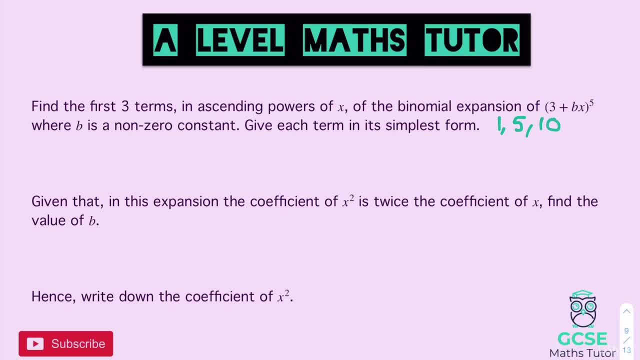 And we've seen this power of 5 quite a lot throughout this video. so hopefully you're recognising that pattern by now: 1,, 5,, 10.. And let's have a look then. our first piece is a 3, and our second piece there is a BX. So let's find these first three terms. So 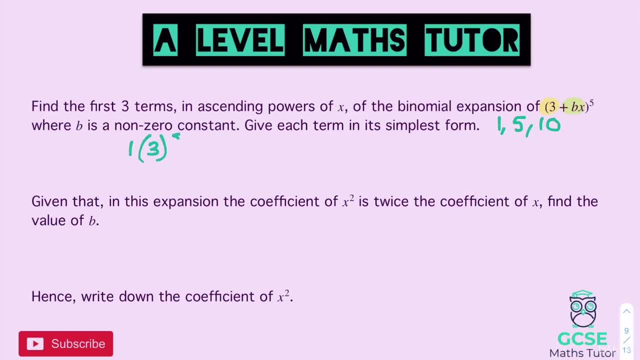 we have 1 lot of the 3 to the power of 5, and then we have 5 lots of 3 to the power of 4, and the BX, and then, for our final piece, we've got 10 lots of 3 to the power of 3. 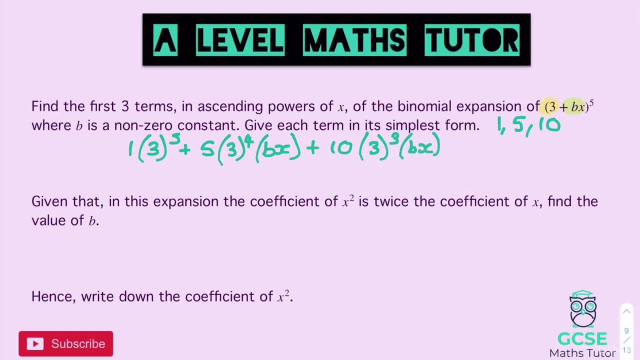 now, and then BX to the power of 2.. There we go, Okay, so simplifying this down. then, 3 to the power of 5 is 243, so we get 243, plus 5C0.. 5 times 3 to the power of 4, which is 405, so plus 405, BX plus 10 times 3, cubed well. 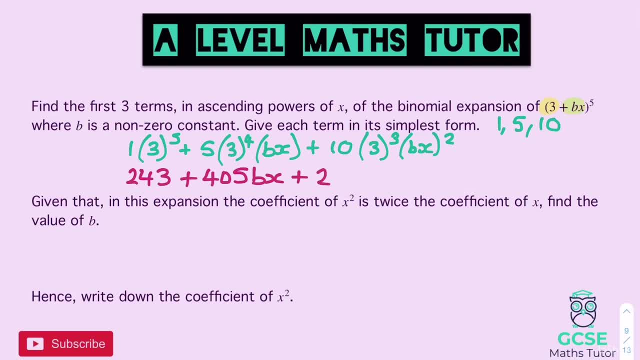 3 cubed is 27,, so times it by 10 is 270,, so 270,, and then squaring BX gives us B squared, X squared, And there we go, and there's our first three terms. So, given that the in this expansion, 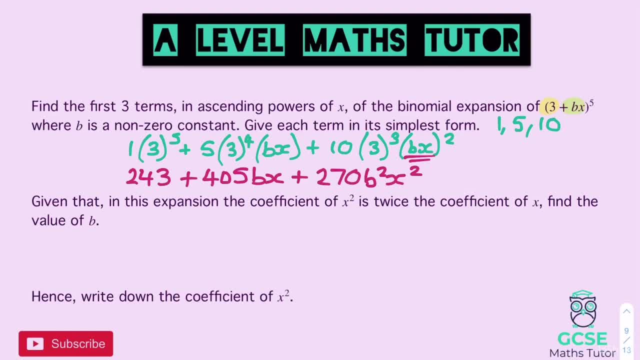 the coefficient of X squared is twice the coefficient of X, find the value of B. So again, completely up to you whether you double one or half the other, but our coefficient of X squared is 270B squared and the coefficient of X is 405B. 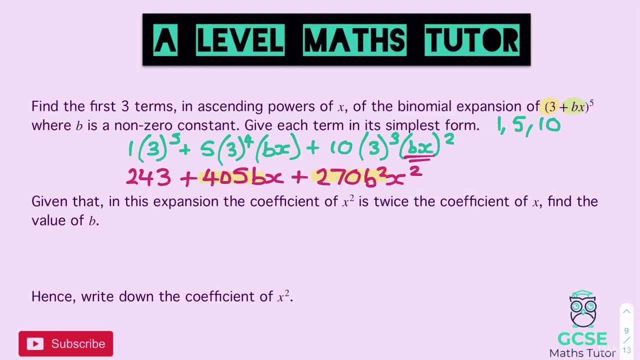 So it says the coefficient of X squared is twice the coefficient of X. So again, completely up to you whether you double one or half the other. I'm going to go for halving this one this time. So we have: 405B is equal to half of that. so 270 divided by 2 is 135, equals 135.. So 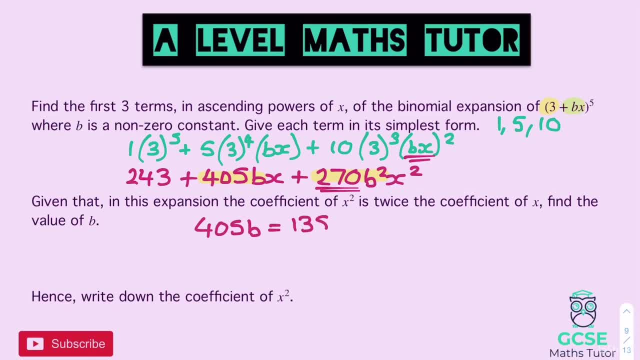 we've got 405B squared. Okay, Divide both sides by B to start with, or however you like really, but we get 405 equals 135B, and then we can divide both sides by 135.. So 405 divided by 135 equals 3, so we get. 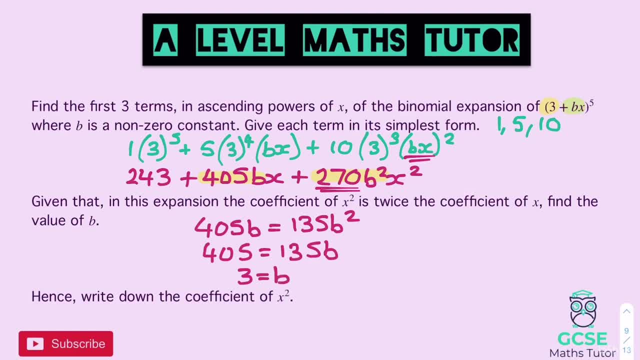 3 equals B, or B equals 3.. There we go, and there's our value of B. Then it says: hence write down the coefficient of X squared. Well, we already know X squared up here We have 270B. squared is our coefficient. 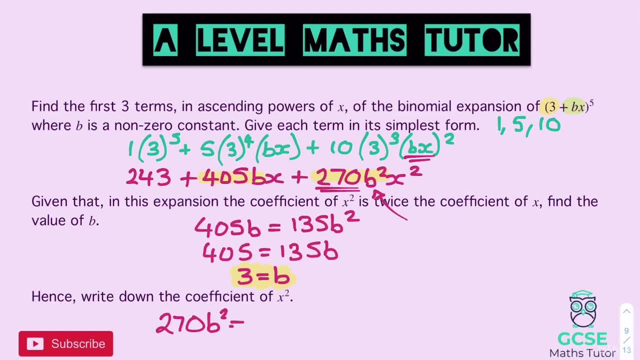 So 270B squared, and if I substitute 3 into that, we get 270 times by 3 squared. So 270 times 9, which is 2430, and there we go. there's our coefficient of X squared in this binomial expansion. 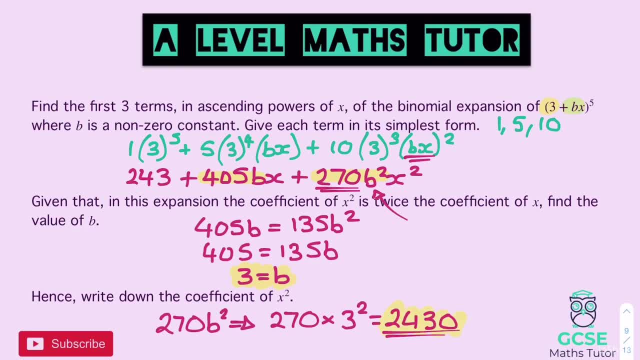 Right, there we go. so that's the final answer for that part. Hopefully, you found that quite nice and simple. Obviously, following some of that process, I've got one more question for you to have a look at before we finish here, so let's have a look at that one now. 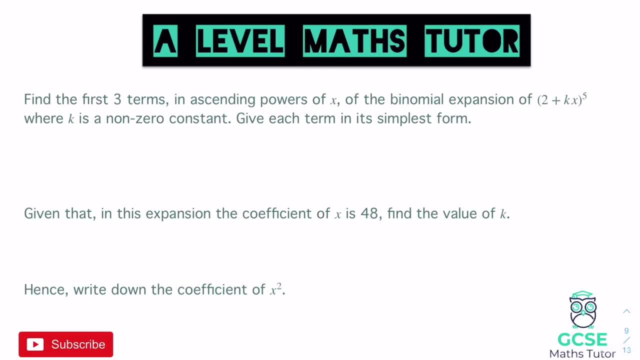 Okay, so this question isn't really any more difficult than the previous two. just another question for you to have a go at, really with some slightly different wording in the second part. there It says: given that in this expansion the coefficient of X is 48, find the value of. 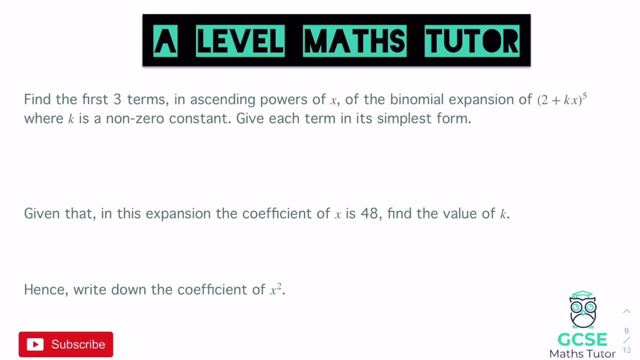 K. So pause the video there, have a read through this, have a go as our last question and we'll go over the answer in a sec. Okay, so the first three terms: notice to the power of 5 again. so we've got our first. 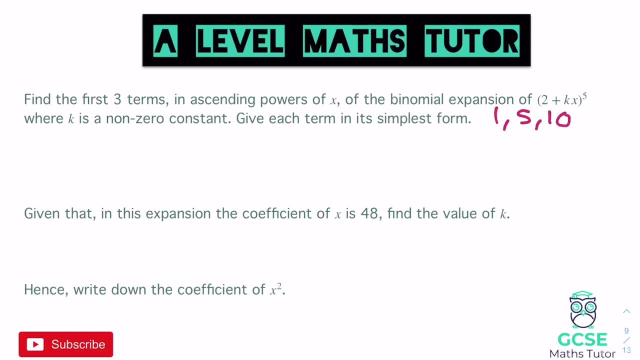 three pieces are 1,, 5, and 10, and we just need to obviously work this out. So our first piece in there is a 2, and our second piece there is KX. So we have 1 lot of 2 to the power of 5, and then we have 5- lots of we've got 2 to the 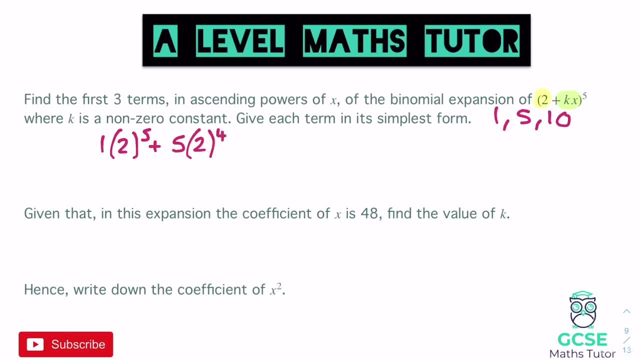 power of 4, and the KX, and then for our final piece, 10, lots of 2 to the power of 3, and then our KX squared. There we go. and if we simplify that, 2 to the power of 5,, let's work that out: 32,, 5. 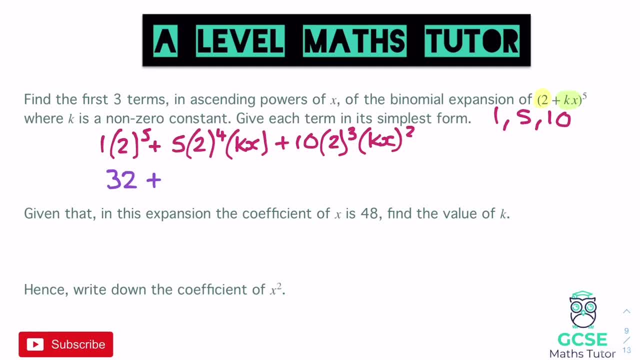 times 2 to the power of 4, let's work that out: 5 times 2 to the power of 4 is 80, so we have 80 KX. 10 times 2 cubed: 2 cubed is 8, so that's 80, so we get 80 K squared X. 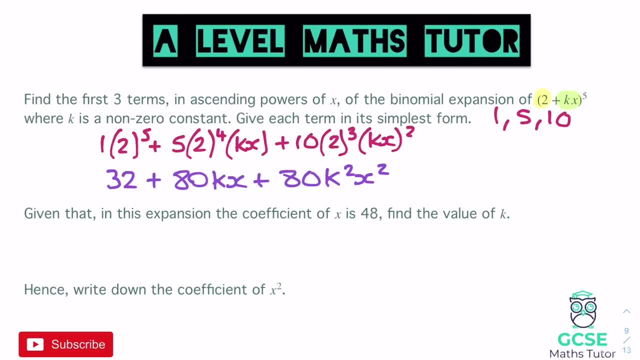 squared. and there we go, squaring KX. Okay, So there's our first three terms. it says: given that in this expansion, the coefficient of X is 48, find the value of K. well, the coefficient of X is 80 K. so it says that. 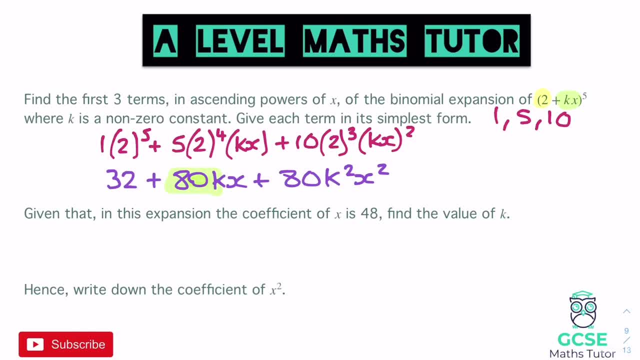 80 K is equal to 48, so if we write that as an equation, we get: 80 K equals 48, so straight away we can just divide both sides by 80, so K is equal to 48 over 80, which if we work, 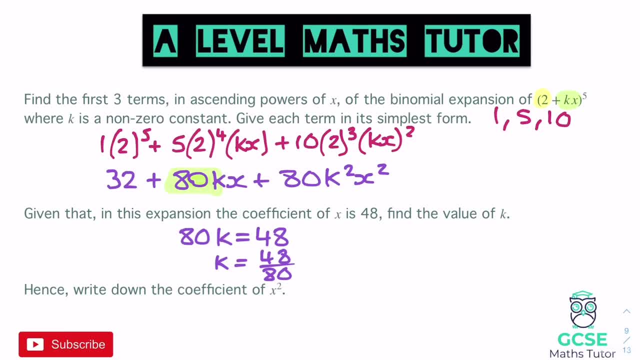 out in the calculator simplifies down to 3 over 5, there we go, which equals 3 over 5.. Or you could write that as 0.6, and then it says: hence write down the coefficient of X squared. well, the coefficient of X squared- let's have a look- is 80 K squared. so we 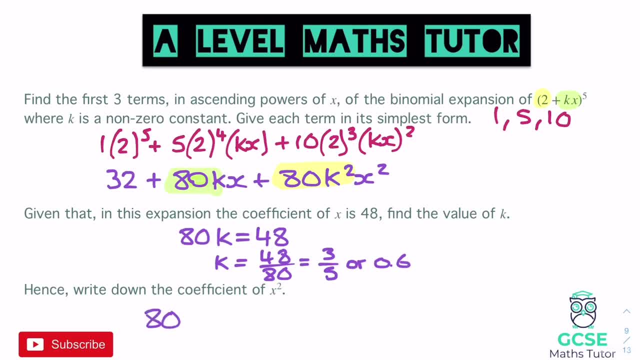 just need to sub that into there. so let's have a look. we get 80 K squared and we know that K is 0.6, so we can do 80 multiplied by 0.6 squared and let's see what we get.